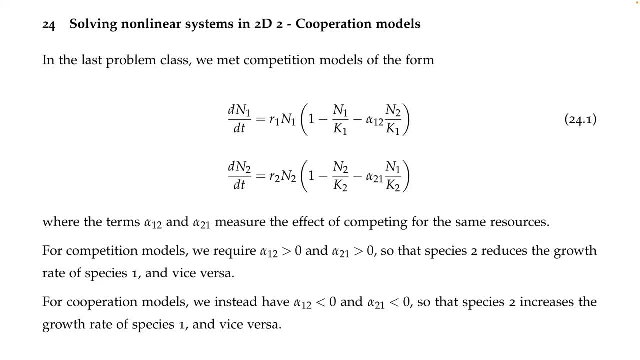 Today is our last lecture on nonlinear systems. Like I said, nonlinear systems are not on this midterm, but they will be on the final. We have been through various different types of nonlinear systems so far. We've looked at predator-prey models. We've looked at disease. 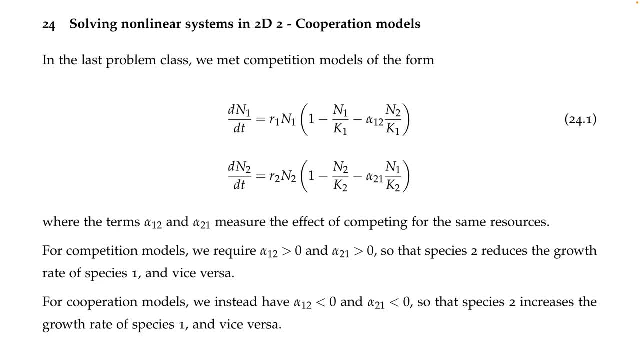 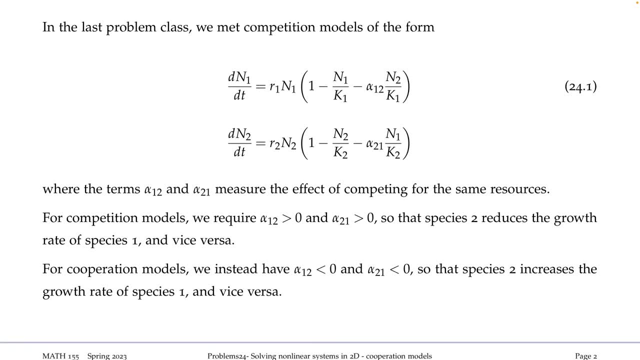 models, competition models last time out, and today we're looking at a variation on the competition models and thinking about cooperation instead. So we're going to be doing basically the same stuff that we've done before: thinking about equilibrium or fixed points, thinking about 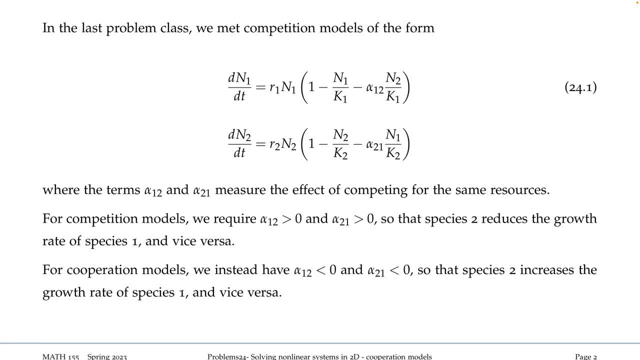 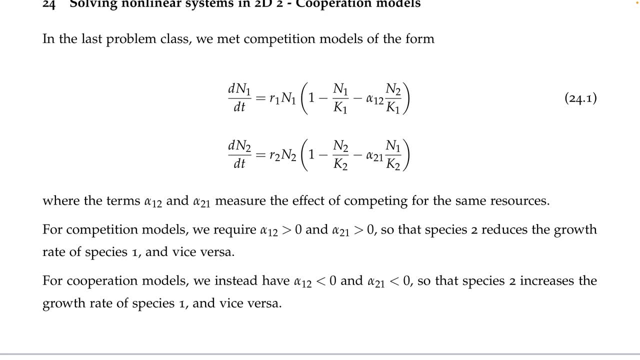 their stability and drawing phase planes. There's a pattern here. There's lots of practice for you guys to work on this stuff. Okay, so last time we met a competition model that looked like this, which is basically a logistic model for two species, and then we had this additional. 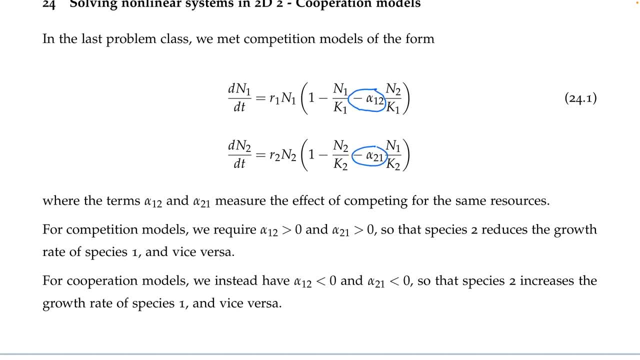 term with these coefficients, these alpha-1-2s and alpha-2-1s. that were negative terms, So they were indicating that there was a negative interaction between these species- competition in this case- And so we had a look at this and the different types of orientations of phase planes that we 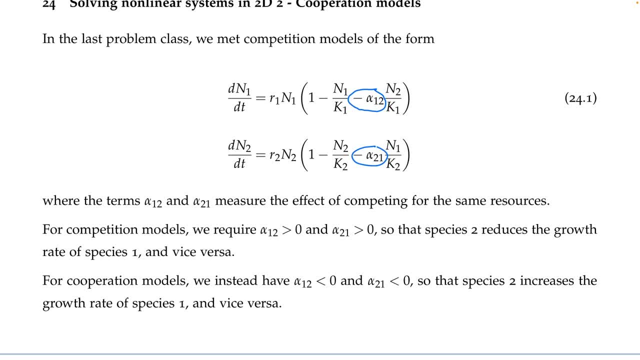 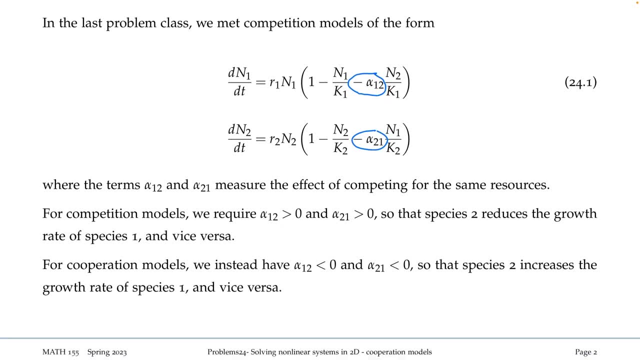 could get and what that would mean for the stability of the system. So could these species coexist or not? When could they coexist or not, Depending on these values here, as well as their carrying capacities. So that's the first thing we're going to be doing. 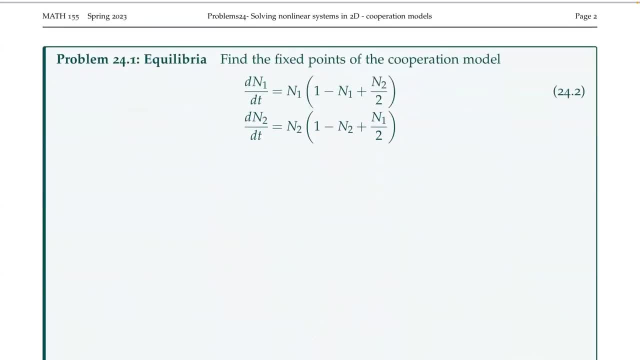 So let's throw it out and see if you're Nobelist. So that was a model where we had negative interactions. Now we're going to think about what happens if we have a positive interaction here. So what does this mean? So, 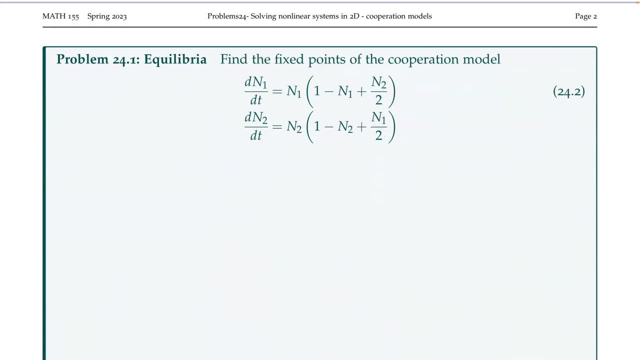 So rather than a competition model we have a cooperation model. So if we just cross out these into sphere-specific interaction terms here, we just have a logistic model for each species. they're independent of each other. So now, if we add in these, 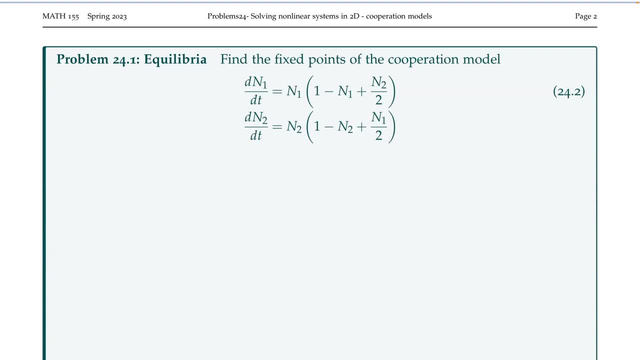 into specific terms here because they're positive. what we're saying here is that N2 is having a positive effect on the growth rate of species one and N1 is having a positive effect on the growth rate of species two. so they're cooperating. so there's lots of examples of this. they've been. 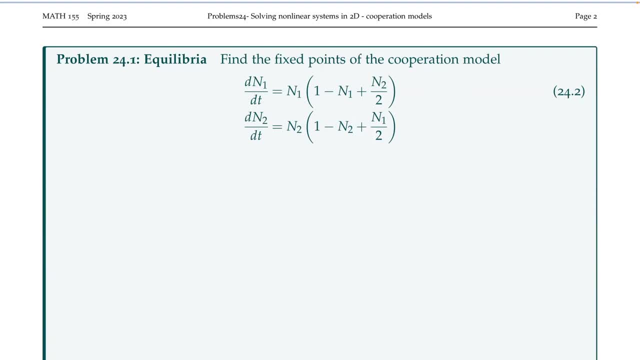 like plants and pollinators, hosts and microbial symbionts, whales and feeder fish- all of these different examples where there's some sort of cooperation between the species. okay, so the first thing we want to do is we want to find the fixed points and then we're going to 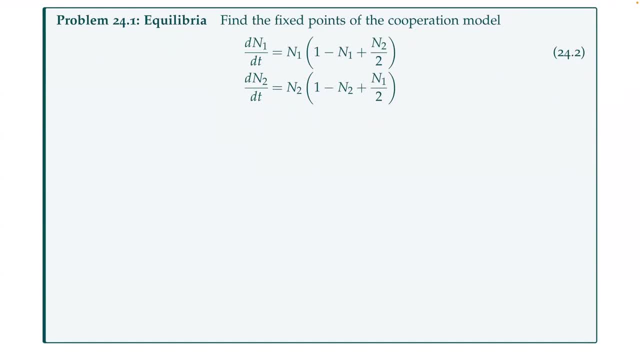 look at the stability. I have a share of hands. who wants me to go through? I'm going to either go through the fixed points or the stability and leave the rest for you guys to practice. okay, so would you guys show of hands? who wants me to go through the fixed points and then give you? 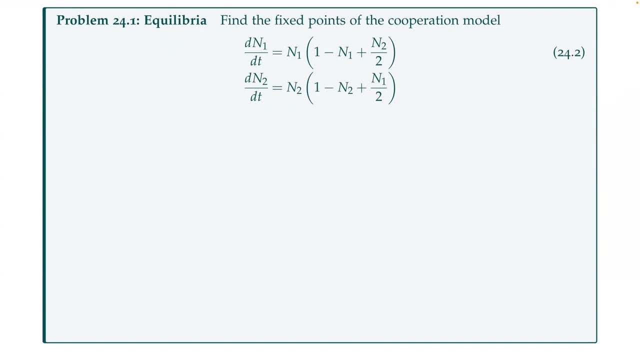 the stability? no one, okay. who wants me to give you the fixed points and wait? which way did I go? let's do that again. who wants me to work through the fixed points? let's show of hands, okay. who wants me to work through the stability instead? right, roughly even, that's great. 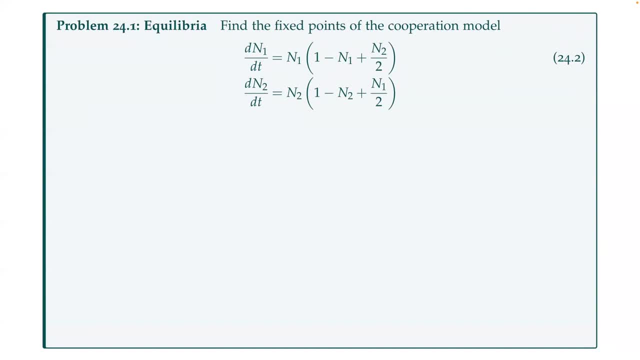 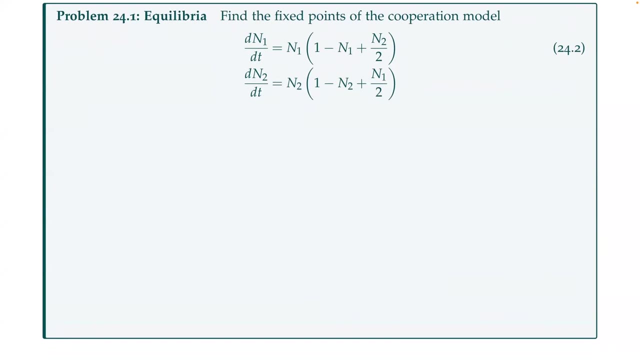 in that case I will. I will go through the fixed points, just to make sure that bit is clear. obviously, the solutions to all of these things will be online and I'll go through the base points as well. so part of the reason I don't want to go through. 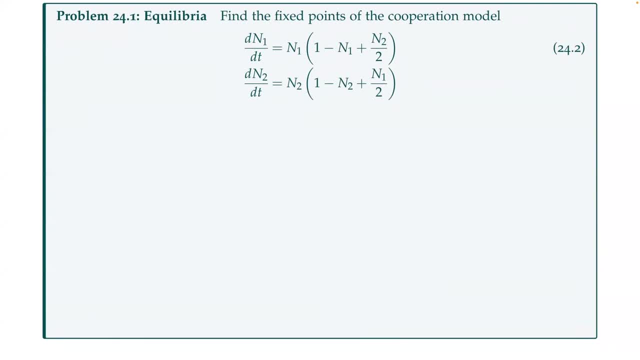 everything is. I want to give you guys some more practice as well, so you can do these things in your own time, okay, so when we're trying to find fixed points, remember what we're doing is: we're going to be setting these equations here equal to zero, and they have to both be equal to zero in order for 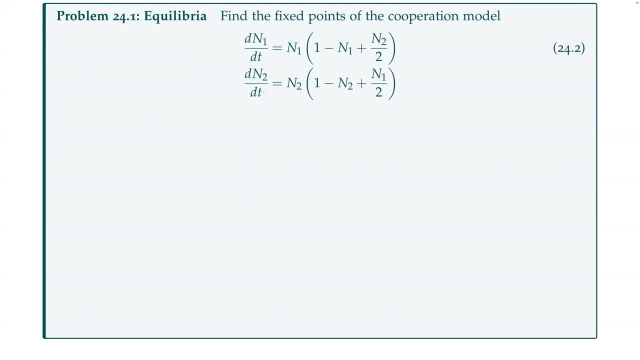 us to get a fixed point. so let's think about the first one. so if we set the n1 dt equal to zero, that means that either we have n1 equal to zero because we have these two, two terms multiplied together to get zero, one or both of them have to be equal zero. 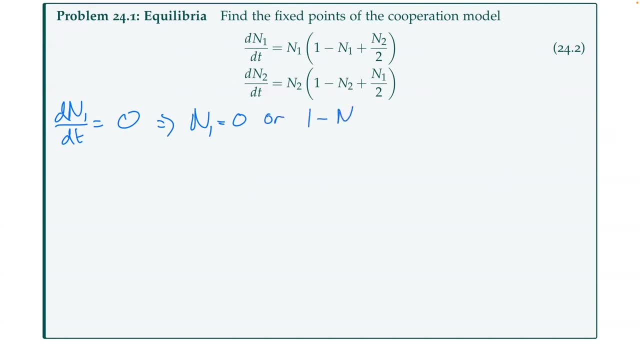 so you either need n1 to equal zero or one minus n1 plus n2 over two to equal zero. we can rearrange this: for n1 we should have one plus n2 over two, so n1 is equal to one plus n2 over two. 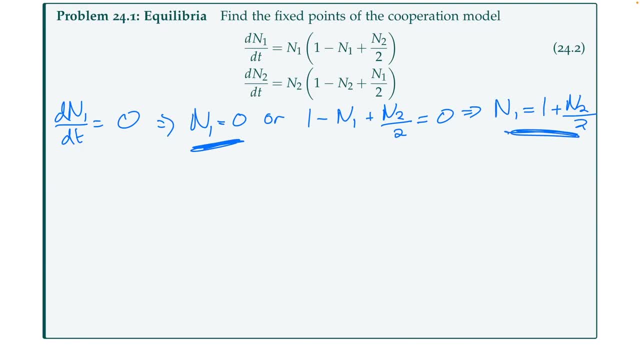 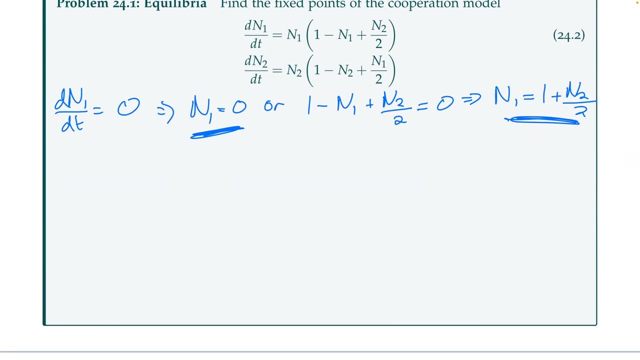 so what this means is we either need this or we need this condition to have the n1 equal to zero back down to zero. two prove: we're still training three n1s to equal zero. so it gives us n2 equal to zero one, and we do the same thing here as well as we want to do if the n1 in bishop2 is equal. 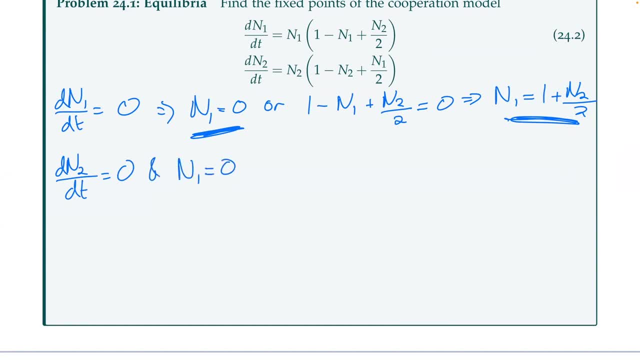 zero, then we're going to increase k1jx by two and working to get that n1k2 equal to zero. how did we do this? one way we can do this is just: let's set the n2 dt to zero and consider what happens if n1 is equal to zero. so this first thing here. 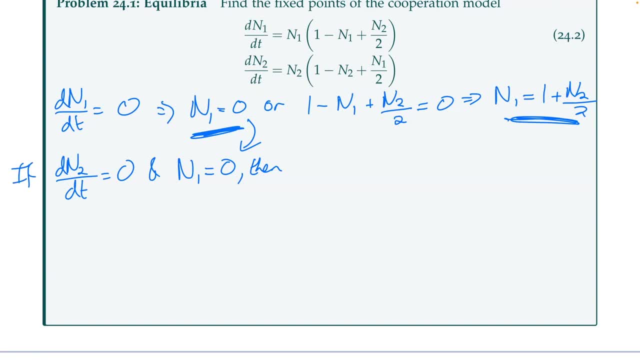 and n1 is equal to zero. Remember, we want both of these things to simultaneously be zero, and above we've got the conditions for when vn1, dt is equal to zero, So we need to self compute those in. So what do we have here? 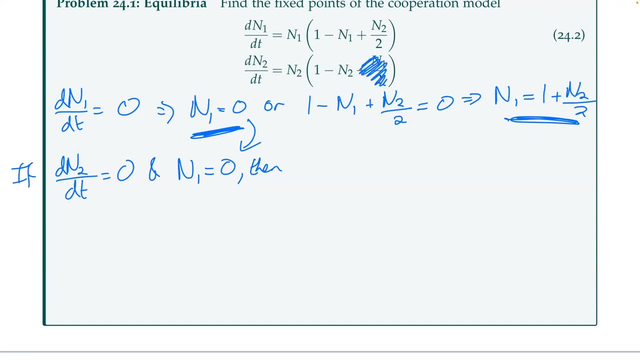 If n1 is equal to zero, then that means that this term here is zero, and this is just our logistic model. So n2 times pi, one minus n2 must equal zero, which implies that n2 is equal to one or n2 is equal to zero. 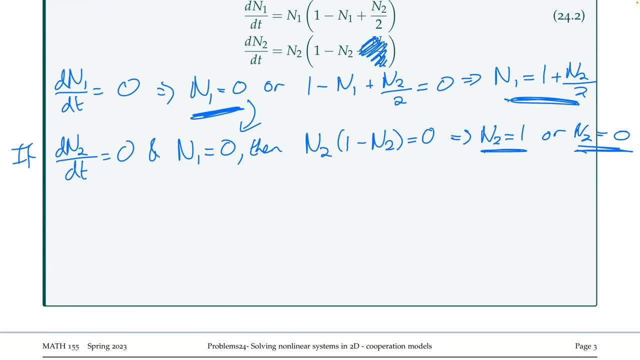 Okay, so for this point I can keep track of what my fixed points are. So I know that I've got a fixed point at zero zero and another one at zero one. Okay, now we consider the other condition in the first equation. 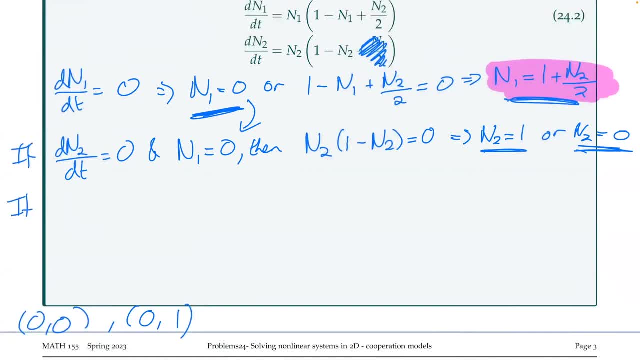 So now we say: if the n2 dt is equal to zero and n1 is equal to one plus n2 over two, then what do we have? Well, in this case we need n2 times pi. one minus n2 plus n1 over two equals zero. 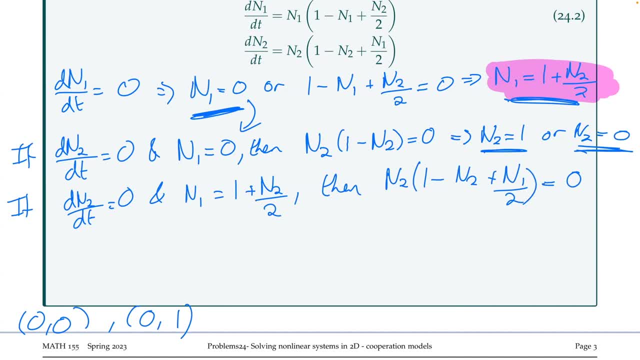 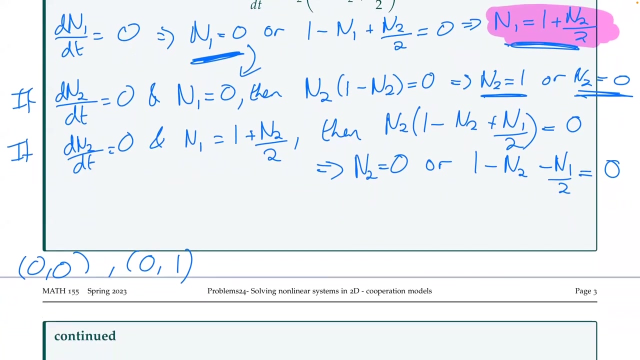 That's just the second equation- equal to zero. So that means that either n2 is equal to zero or the bit in the brackets one minus n2 plus n1 over two is equal to zero. So again we've got another fixed point here already. 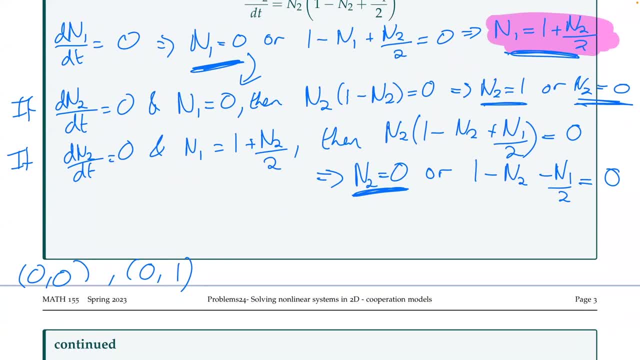 If n1 is equal to 1 plus n2 over 2, then either we need n2 is equal to 0 or this second condition here on the right to be equal to 0. If n2 is equal to 0, we can substitute it back into here. 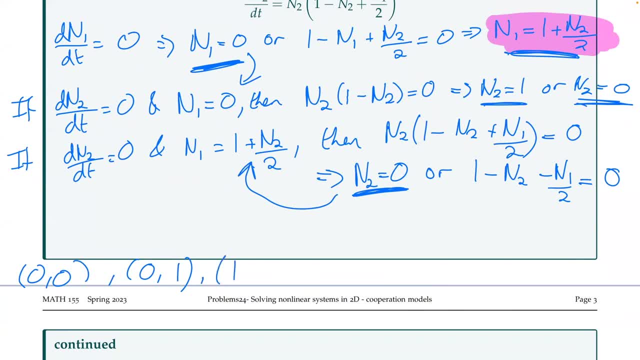 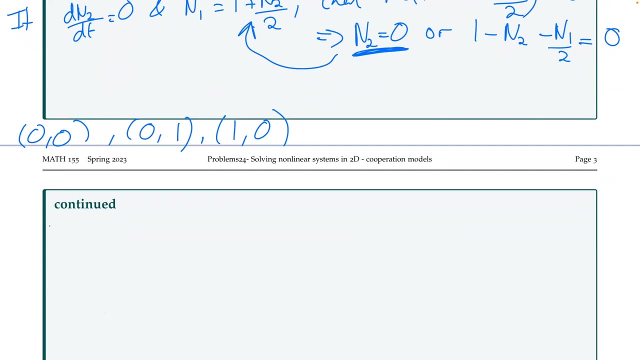 That's going to give me, n1 is 1 and n2 is 0.. So the final ones. we've got three of our fixed points so far. There's a fourth one here. So if we have 1 minus n2 minus n1 over 2 is equal to 0,. 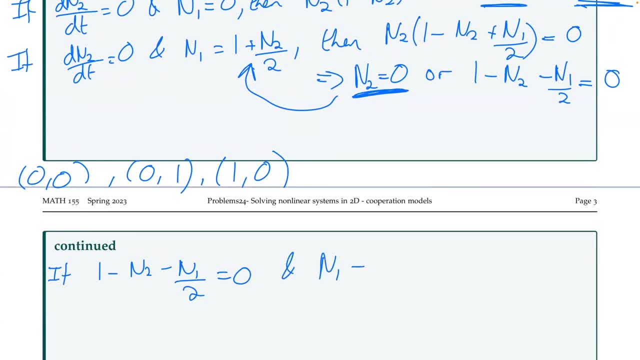 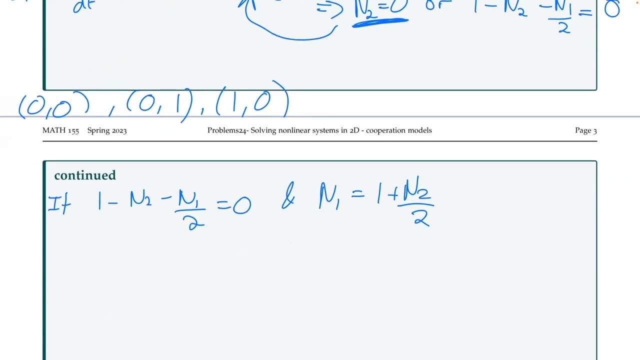 and remember we had to start with: n1 is equal to 1 plus n2 over 2.. We've got two equations. We've got two equations. We've got two equations here and two unknowns. We just need to solve these. 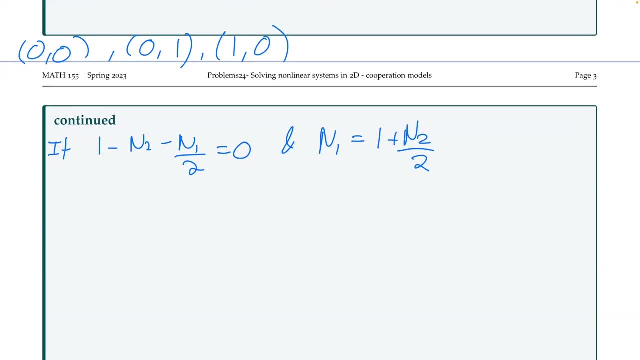 In fact, this is a linear system. You could put this in a linear system and solve it using matrices, like we had previously. So let's rearrange this and substitute this into here We are going to have- let's see, we're going to have a 1 minus n2 minus n1 over 2.. 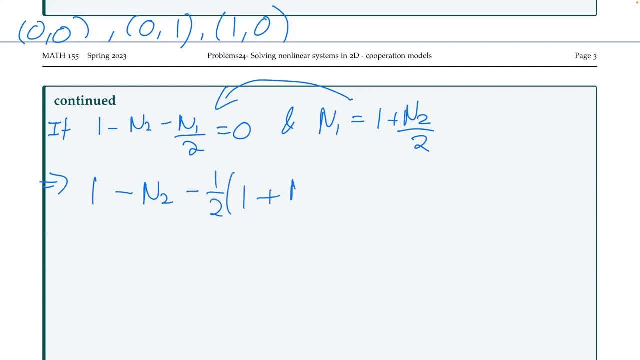 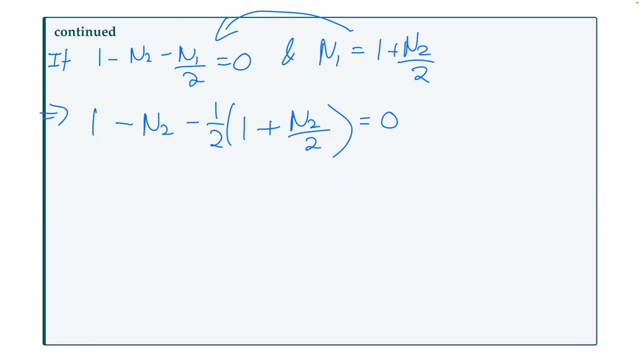 So let's take this half out the front, We're going to have 1 plus n2 over 2.. That's going to equal 0.. Let's expand those brackets. 1 minus n2 minus a half, minus n2 over 4 is equal to 0.. 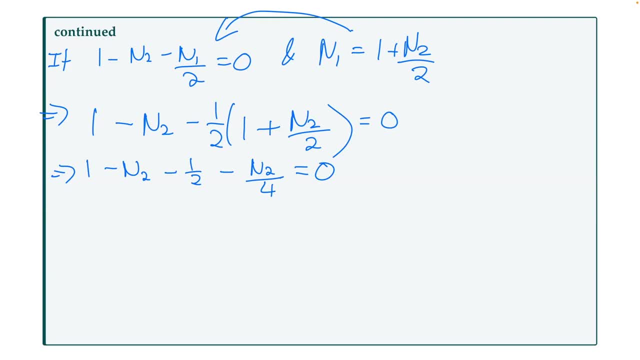 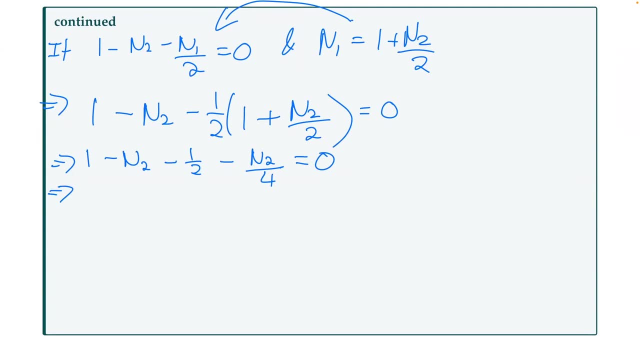 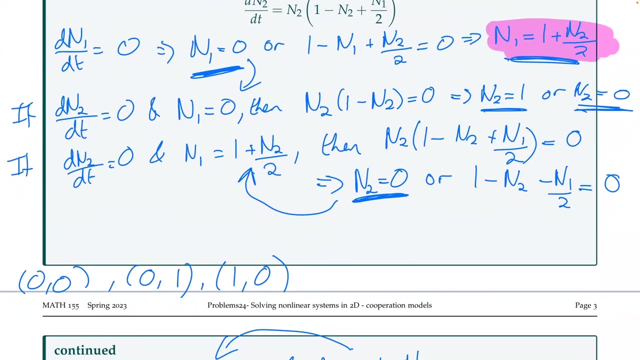 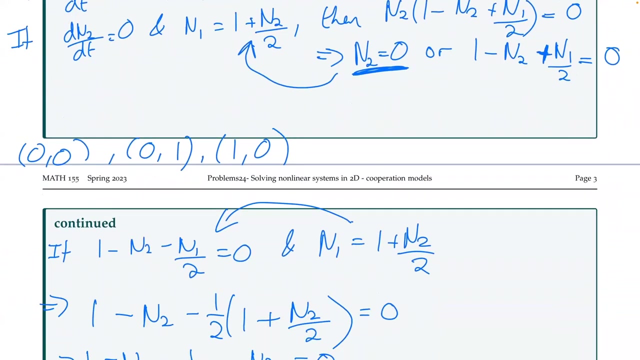 1 minus n2 over 4 is equal to 0.. Let's repeat this. I've got a mistake here. That's because I've got an additional plus. sorry, I said minus n1 over 2.. I'm thinking of my competition model. 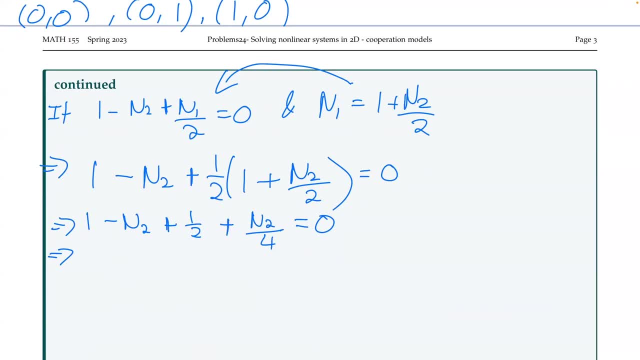 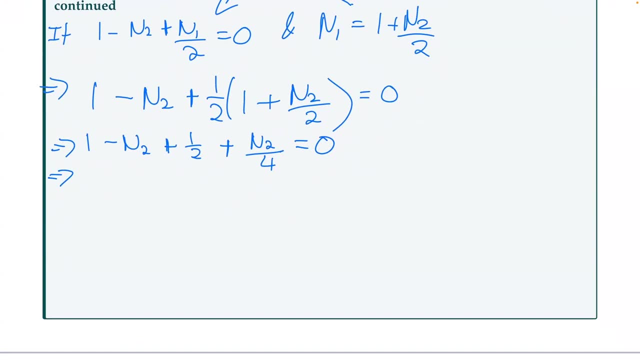 that should have been a plus n1 over 2, which makes this a plus n1 over 2, which makes this a plus. I will work a lot with competition models. this is a positive interaction, which is why we've had a positive sign here, not a negative sign. 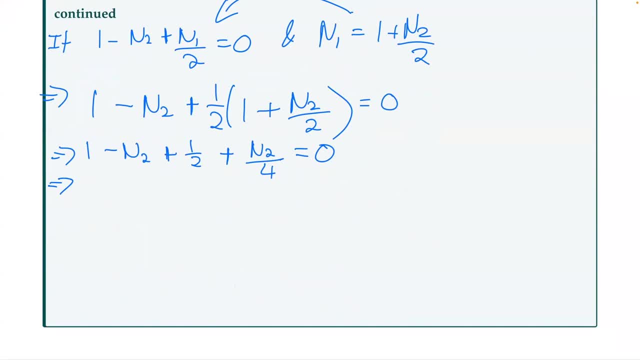 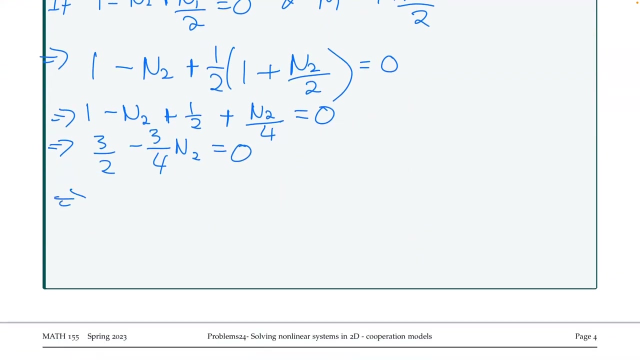 okay, let's see where we're at. so we've got a one plus a half, so it's going to be three over two. we've got minus n over two plus a quarter of n over two, so that's going to be minus three quarters n two, zero. so this just simplifies to be n two is equal to two. 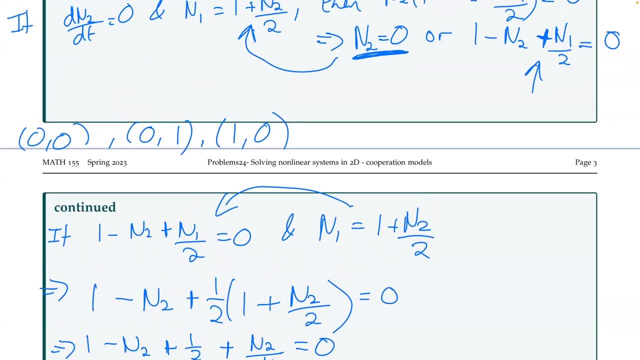 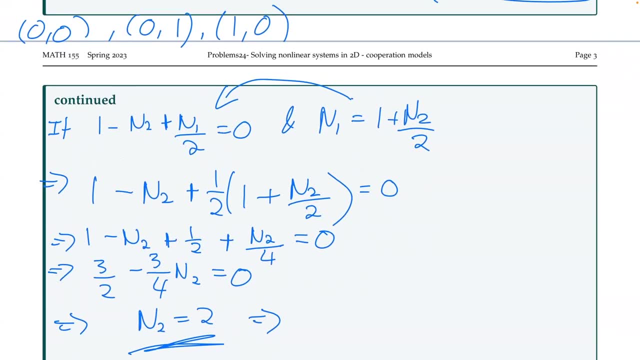 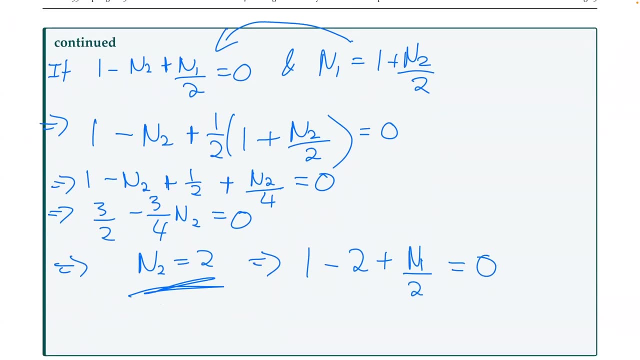 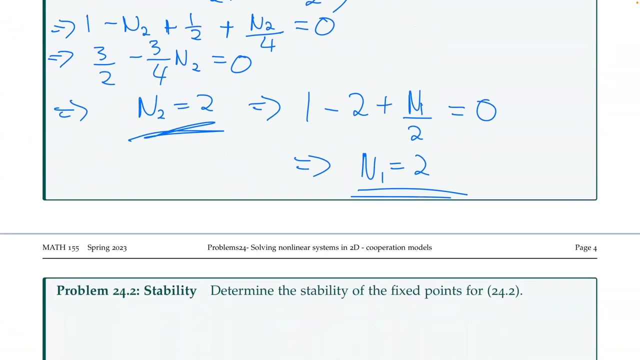 if n two is equal to two, we just substitute it back into this thing up here. so we had one minus two plus n. one over two is equal to zero. so we can rearrange it to be n. one is equal to two. so this means that we have four equilibrium or four fixed points. 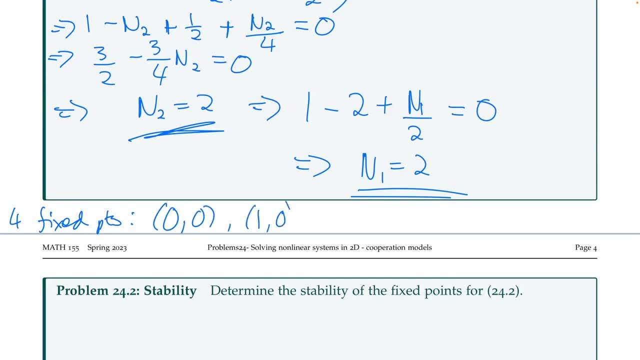 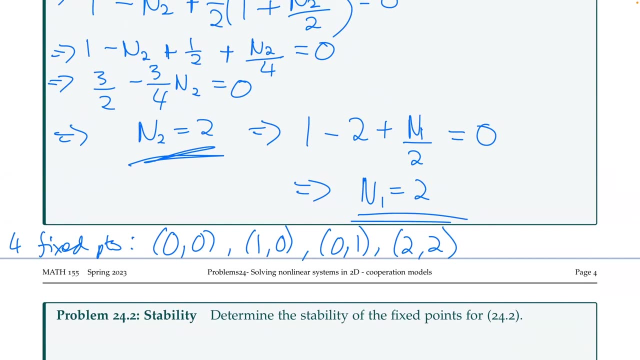 zero zero, one, zero zero one and two, two. you might see these referred to as zero zero being a trivial equilibrium. it's trivial because if this is a positive sign, it's not going to be a negative sign- population model- and if there's no individuals in the population, then obviously nothing's going to. 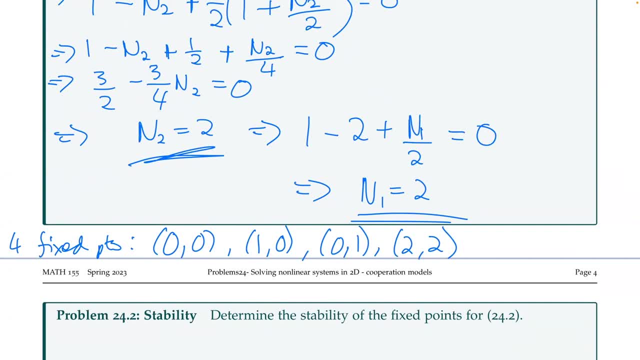 change. one zero and zero one are often called semi-trivial equilibria because there's only one species there. so it just this two species model collapses to a one species model. it's just the logistic model with one species. that's why it's called semi-trivial. and then this last one. 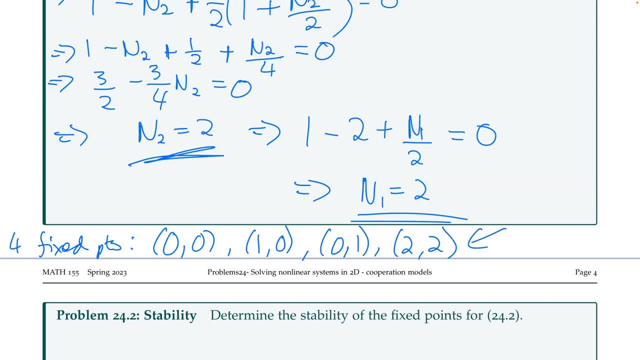 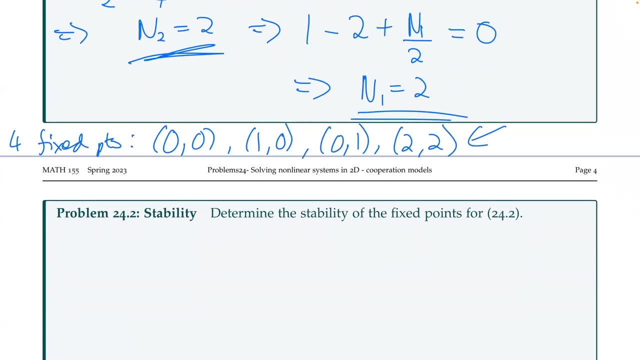 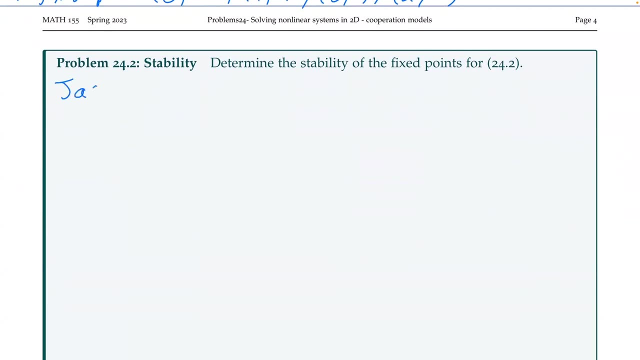 here is often called a non-trivial or a coexistence equilibrium, because both of our species are present. we don't know anything about the stability of that, though. okay, so how do we work out stability? well, we need to look at our Jacobian. this Jacobian j is a function of n1 and n2. sometimes we don't put those n1s, n2s in there. 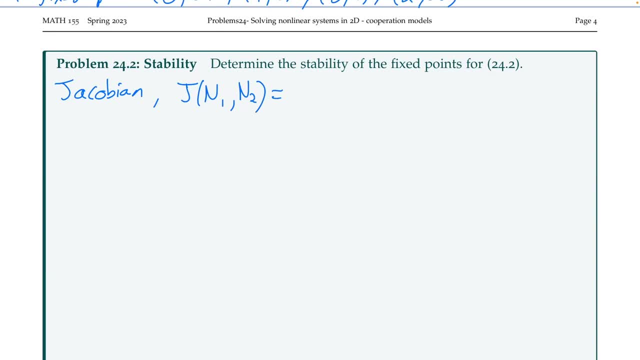 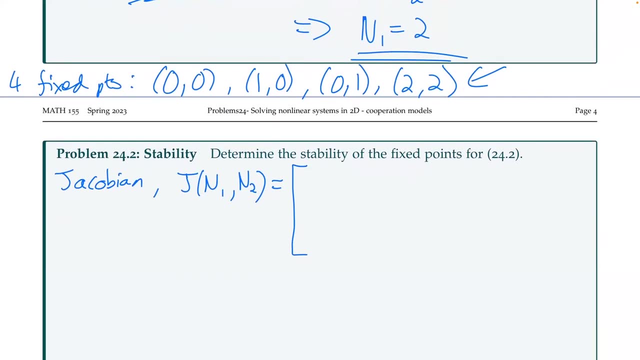 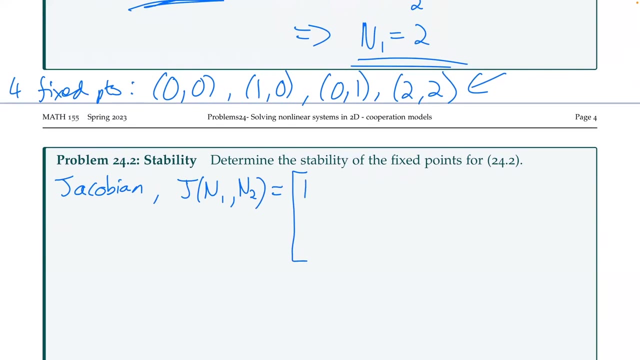 because it's implied, but I'm just including them there to make sure it's explicit here and here we're taking our Jacobian as our matrix of partial differentials, of our partial derivatives, of our functions dn1 dt and dn2 dt. so for dn1 dt, if we take this partial with respect to n1, we get 1 minus 2n1 plus n2 over 2. 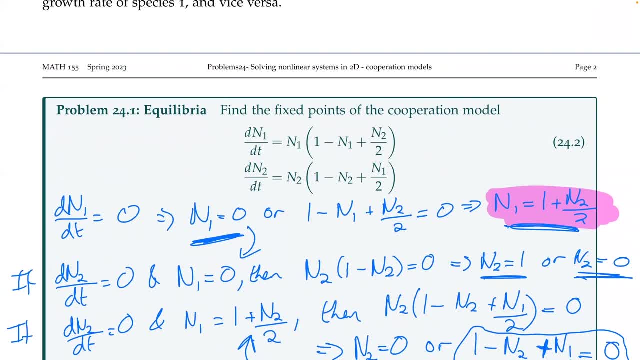 if you're in this sort of situation- before I go on here- and you're not comfortable with taking the derivative when it's in this form, just expand the brackets out, okay. so if I expand these brackets out, I have an n1 minus n1 squared, plus n1, n2 over 2. likewise here I'll have an n2 minus n2 squared. 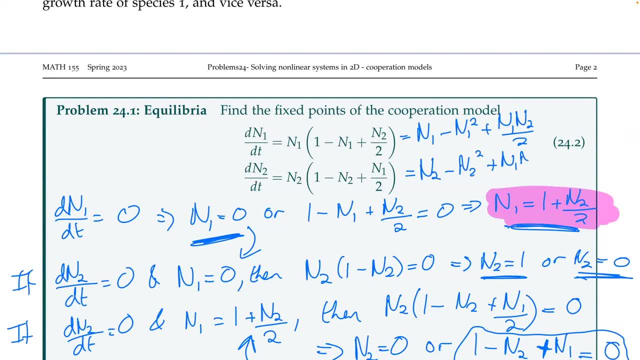 plus n1, n2 over 2.. I think in the solutions I've got a minus here, but that's supposed to be a plus. hopefully I'll remember to correct that. Okay, if you're, if you're in this situation, you don't want to calculate? 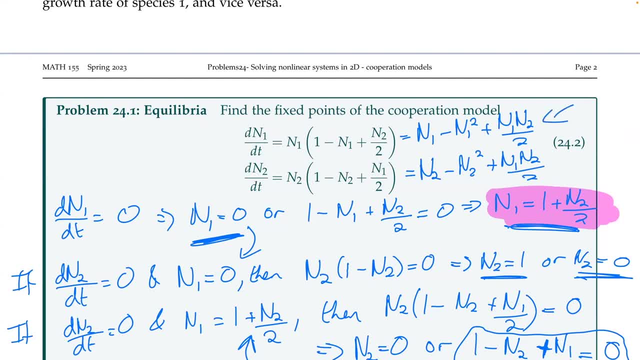 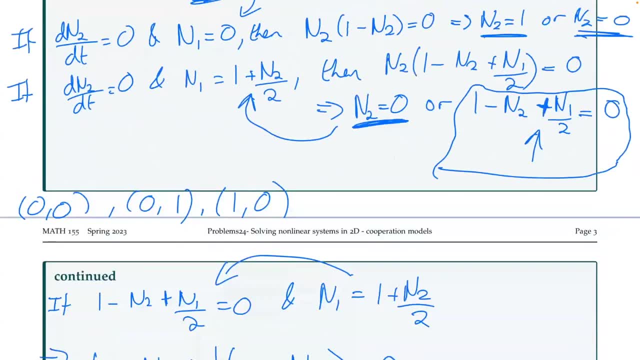 your derivatives directly from here. Just expand the brackets like I've done that. They're all just power laws here, so they're nice and easy to take the derivatives of: Okay, the second partial with respect to n2 here is going to be just n1 over 2.. 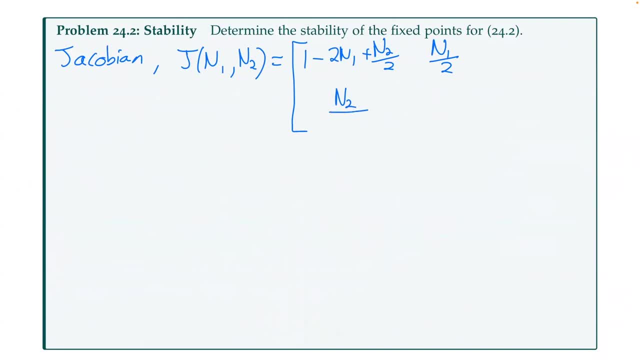 And this system is symmetric, So I can immediately write down what the other partials are, just by changing my n1s and n2s, switching the order of these things around. So in the bottom right I have 1 minus 2n2 plus n1 over 2.. 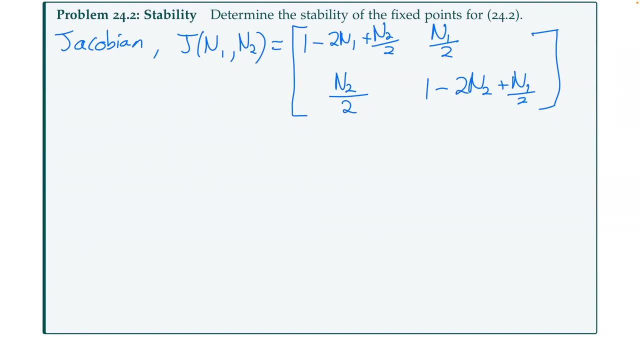 Okay, so I've got my four fixed points, I've got my Jacobian. Now I just need to substitute those fixed points one by one into my Jacobian and either read off my eigenvalues or look at the trace and determinant and then figure out what the stability is. 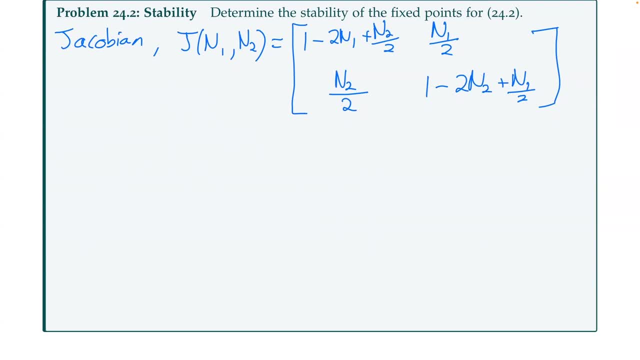 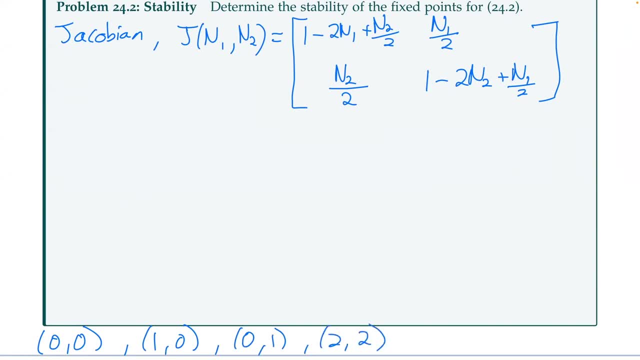 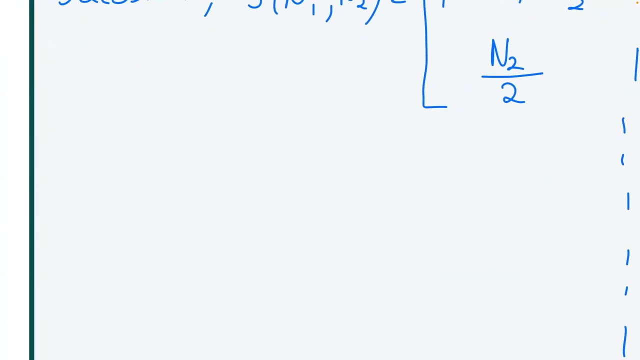 0,, 1, and 2, 2.. Okay, let's see how you guys got on. So our first equilibrium was our trivial equilibrium 0, 0.. So, at 0, 0,, what do we have? 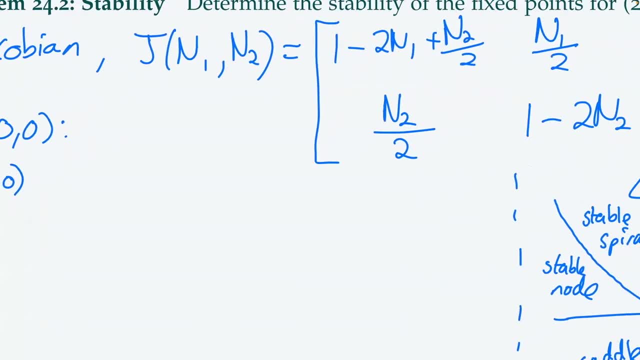 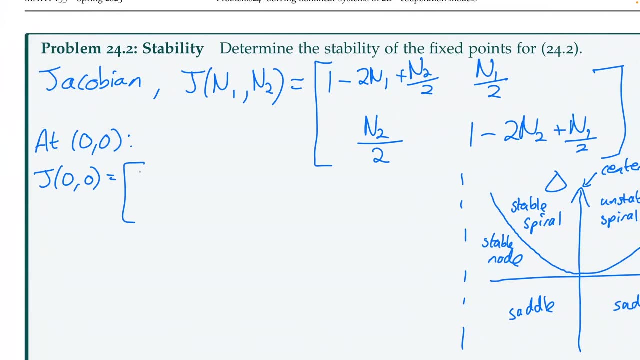 Well, we substitute this into our Jacobian, Our Jacobian. here We're going to have all the n1 and n2 terms are going to be 0. So we're just going to be having 1, 0,, 0,, 1.. 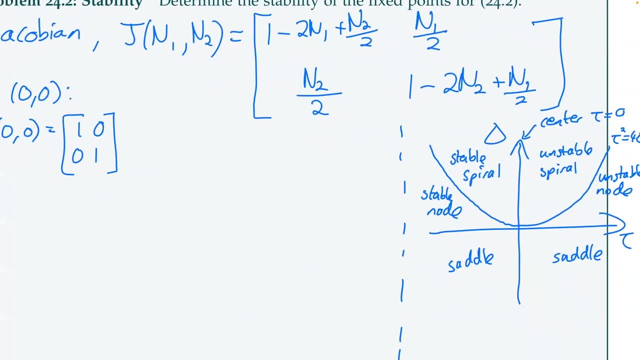 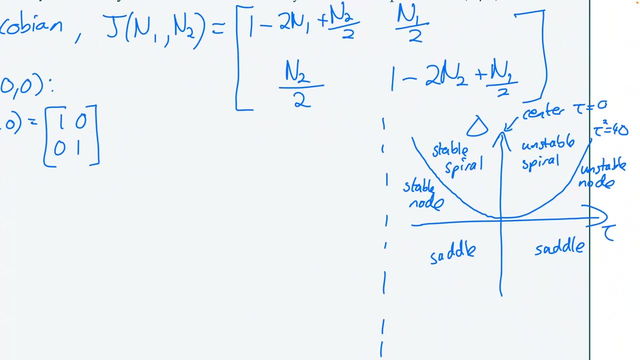 So we could look at the trace and the determinant here. If I look at the trace, I'm going to have a trace of 1 plus 1, which is 2.. That puts me on the right-hand side of this diagram. This is just a sketch of the diagram. 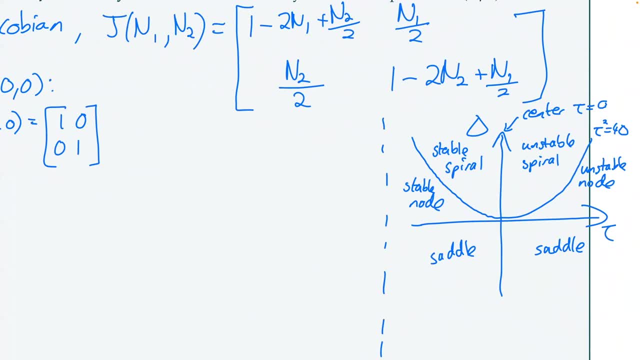 that I've shared with you guys previously. So you'd have a positive trace. Another determinant would also be positive. We could look at our trace. We could look at our trace. We could look at our trace. We could look at our index squared. 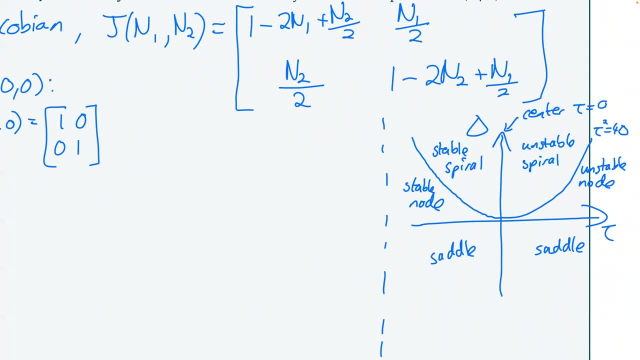 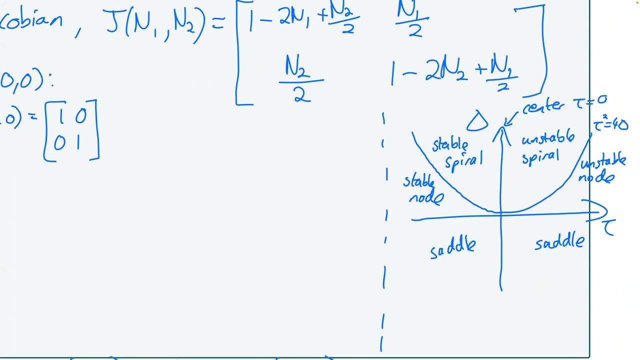 minus four times the determinant, to also work out whether we got an unstable spiral or an unstable node. have an unstable node here. So the other thing we could do is- because this is in diagonal form, So remember- if we have a zero in this place. 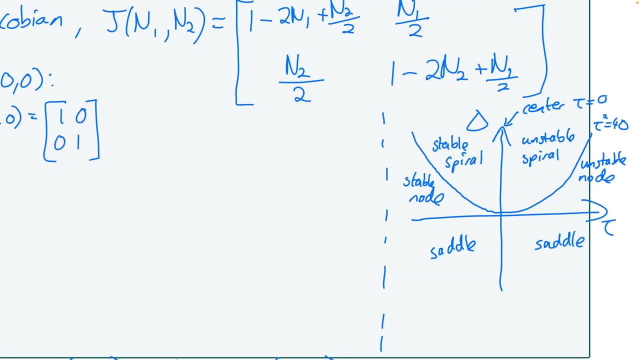 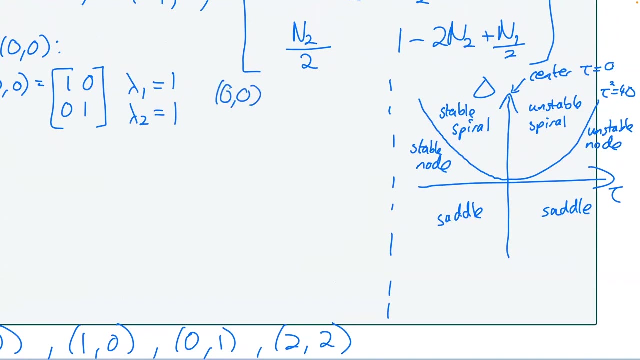 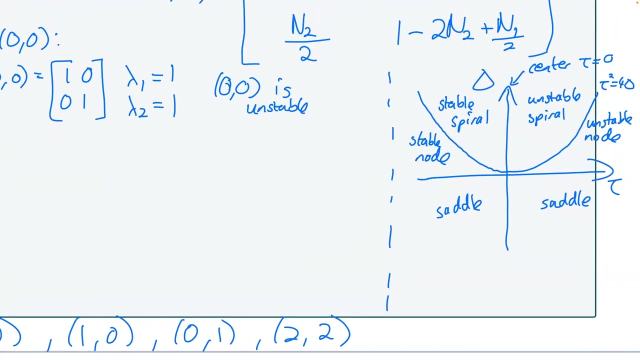 or in this place we can immediately read off our eigenvalues. So in this case, one of my eigenvalues is one, The other one is also one, So 0, 0 is unstable. If you'd worked out the trace. 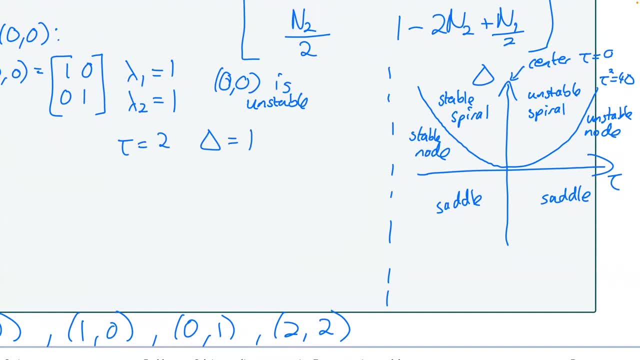 this would have been 2, the determinant would have been 1.. In this case, what we do? take the triplet squared minus four times the determinant, You'd end up with four minus four, which is equal to 0.. So this is one of those cases. 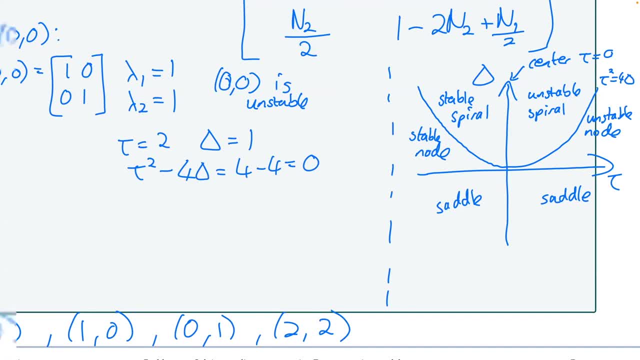 that is on the borderline. This is actually something called a star. So you're actually on this curve here. That is a borderline case here. If this was to appear in an exam, I would just expect you to say unstable. I wouldn't, We won't get into stars. 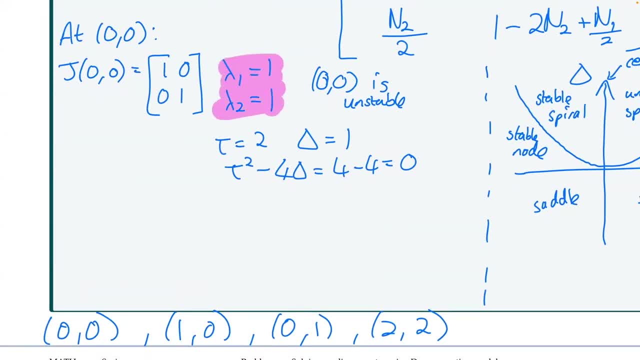 The reason it's a star is because we have these repeated eigenvalues here. That's a bit beyond this course. What I really care about here is whether it's stable or unstable. So in this case it's unstable. That's all I care about here. 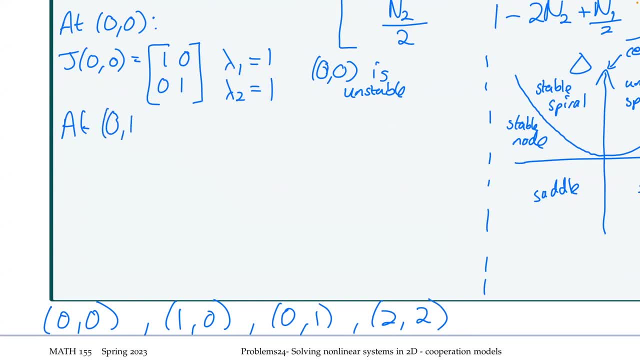 Okay, At 0, 1.. J at 0, 1 is going to be 1 minus a half, 0, a half 1 minus 2, which is a half 0, a half minus 1.. 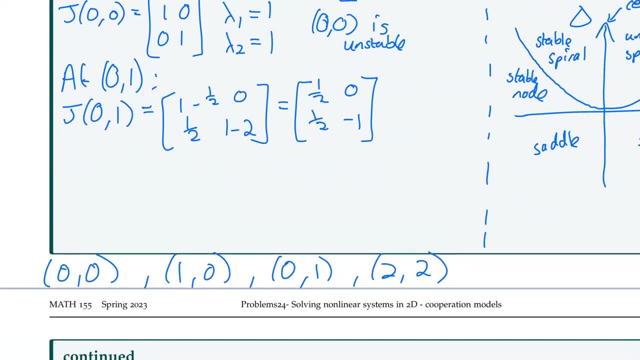 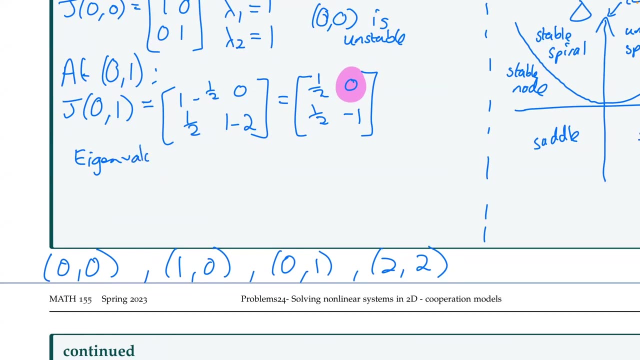 Again because we've got a 0 up. here we're in lower triangular form this time for our matrix. That means our eigenvalues. here we can again read them just off: elements on the main diagonal We have: Lambda 1 is equal to a half. 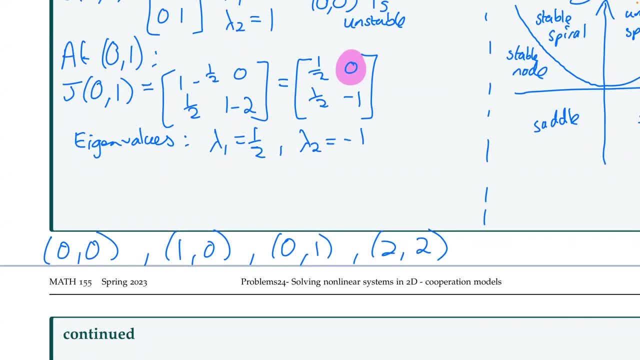 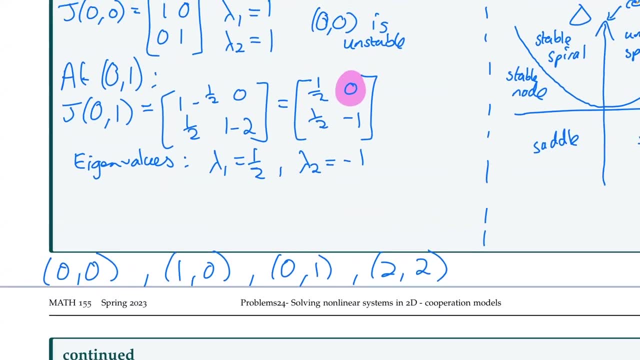 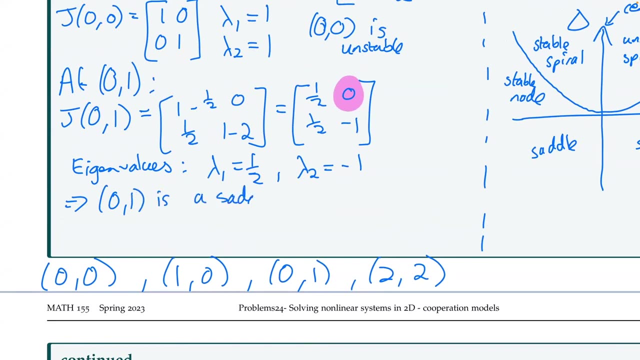 Lambda 2 is equal to minus 1.. So if you remember what it means for your eigenvalues to be positive and negative- if one of them is positive, one of them is negative- that means you have a saddle. Alternatively, if you take your work out, your trace, 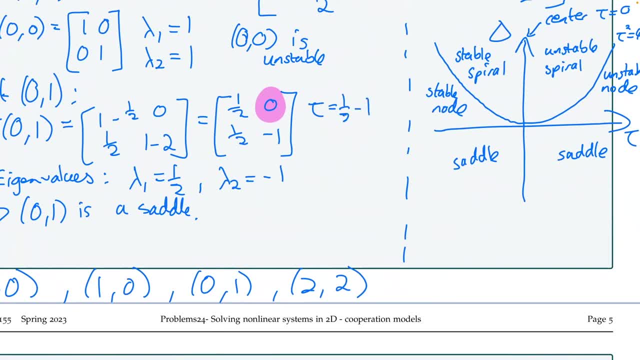 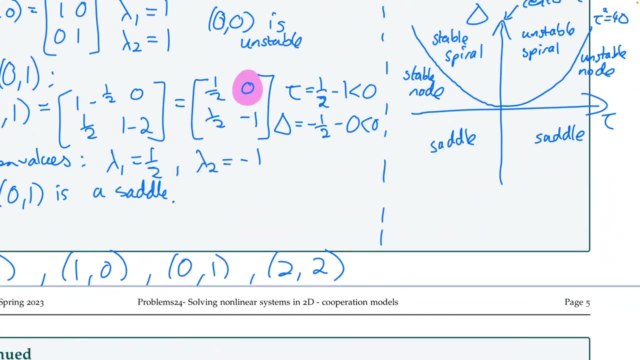 your trace is going to be equal to a half minus 1,, which is less than 0.. Your determinant is going to be minus a half minus 0,, which is less than 0.. So you're in the bottom region of the graph. 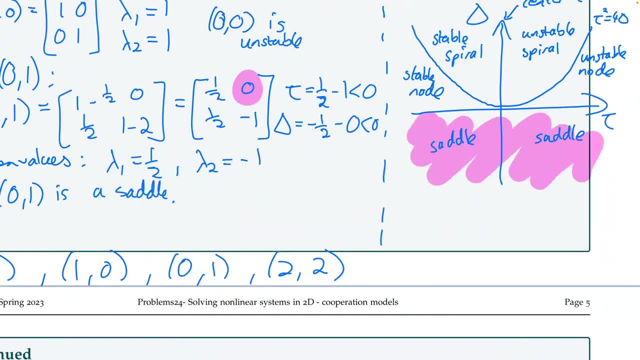 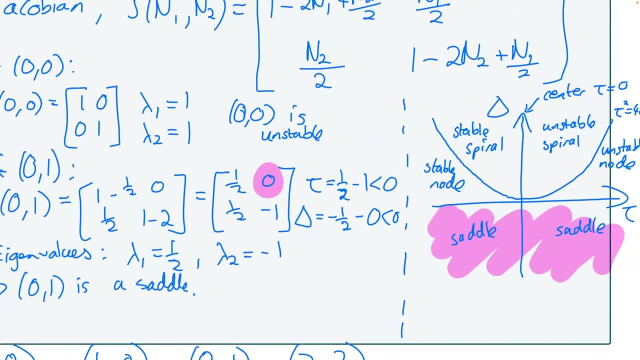 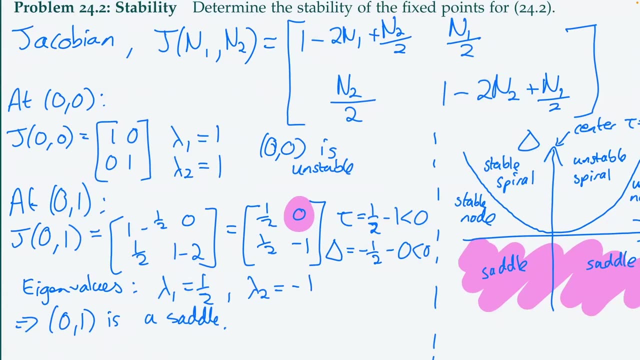 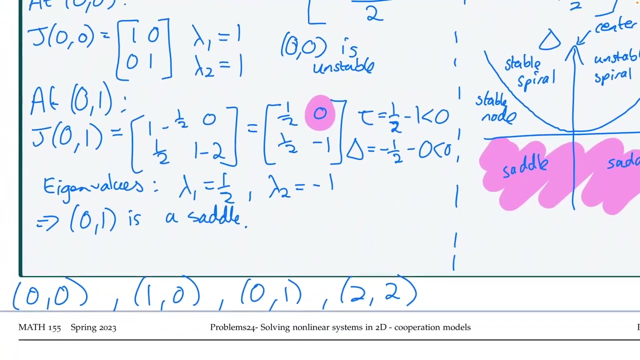 the diagram over here. You have a saddle Question. yeah, Let's see. Yes, it should be 3 over 2, I think I think I just copied that down correctly. So Oh, I think it's because I started doing the 1, 0 instead. 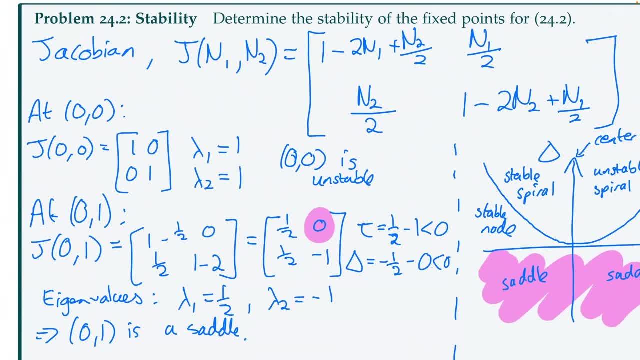 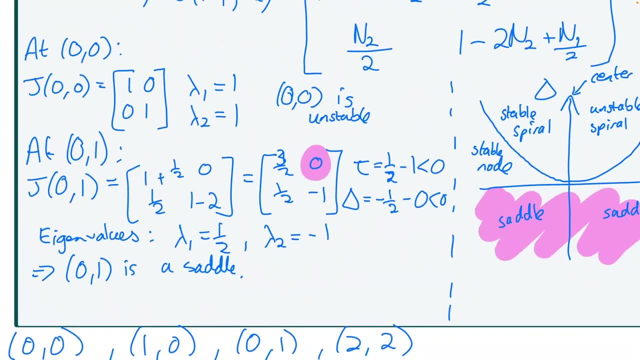 So, yes, n1 is 0. And then you add on a half here, So this should be correct. That should be 3 over 2.. That doesn't end up changing any of the. that changed the sign of this, but that doesn't matter. 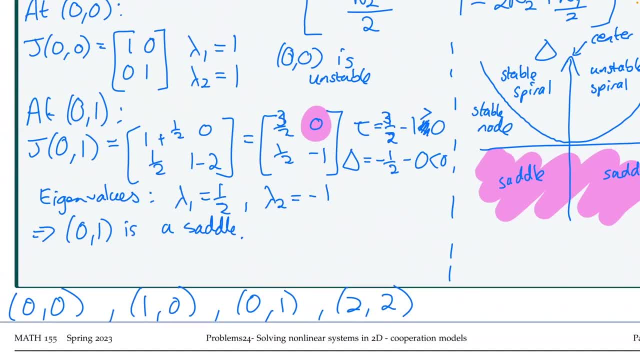 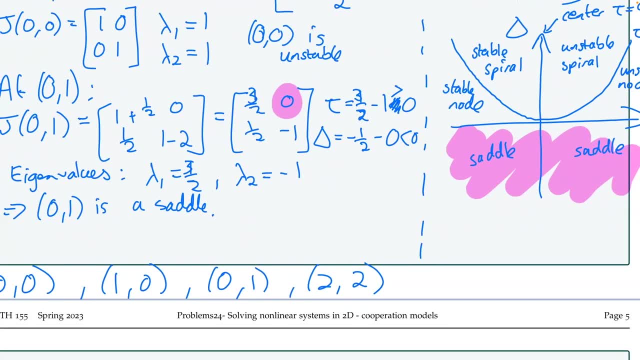 That should be greater than 0. The eigenvalues here have 3 over 2 minus 1.. So it doesn't change the stability of anything. But thank you for spotting that. Again. I'm slipping back into my competition models. Okay, so we have 0,. 1 is the saddle. 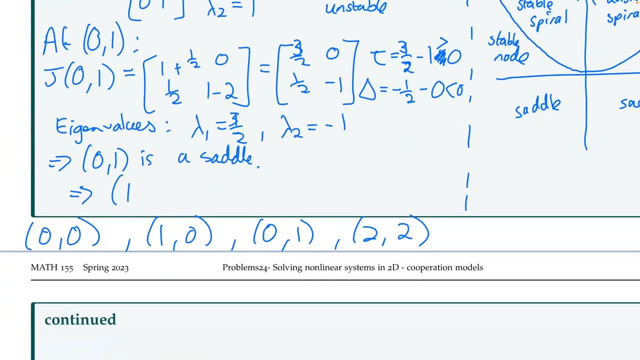 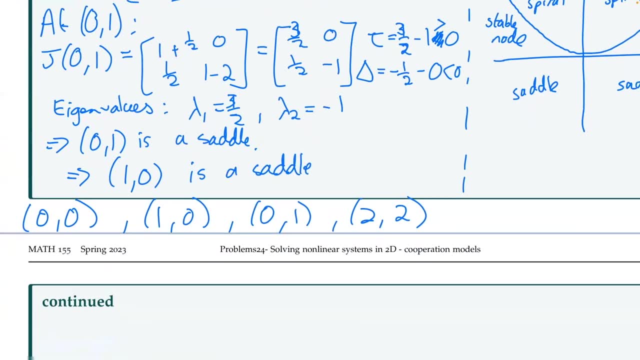 Because this system is symmetric. we can also say that 1, 0 is also a saddle. I'm not going to repeat that. You can work that one out if you want, but it's going to be exactly the same, just flipped around, because this system is symmetric. 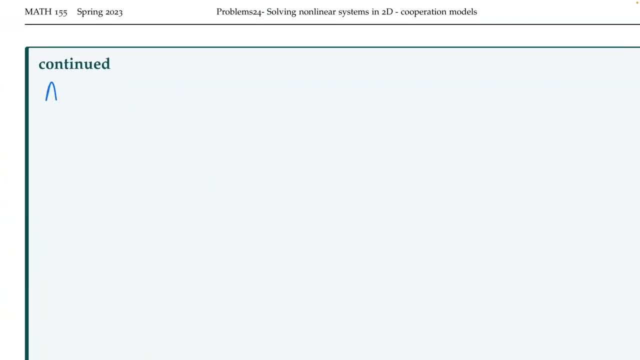 Okay, let's think about our coexistence equilibrium. So at 2, 2, Jacobian, this time it's going to be 1 minus 4 plus 1,, 1,, 1, and again 1 minus 4 plus 1.. 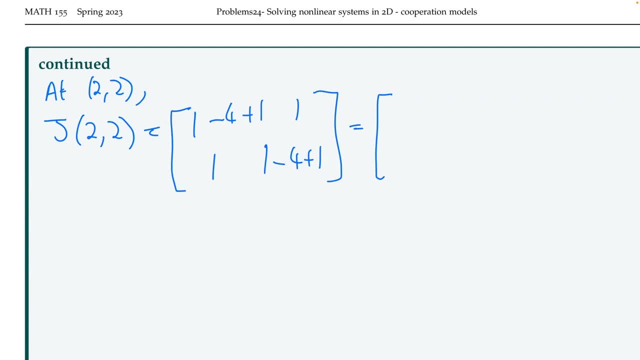 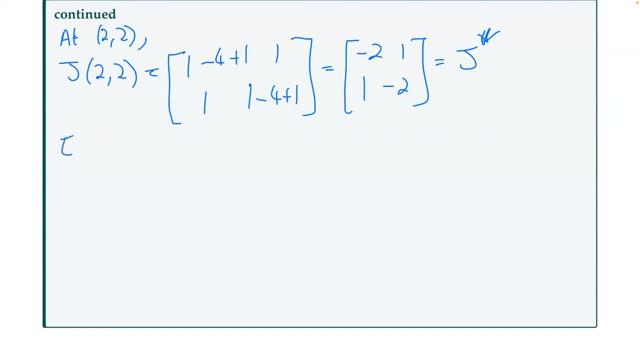 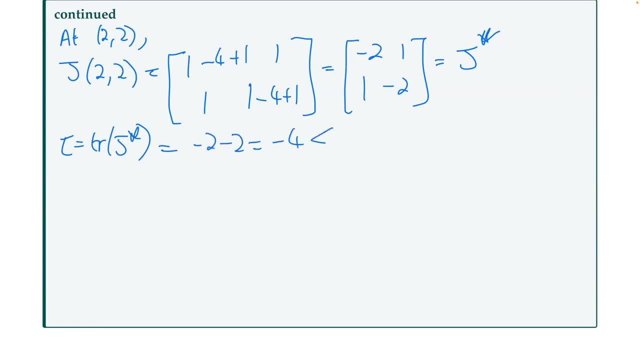 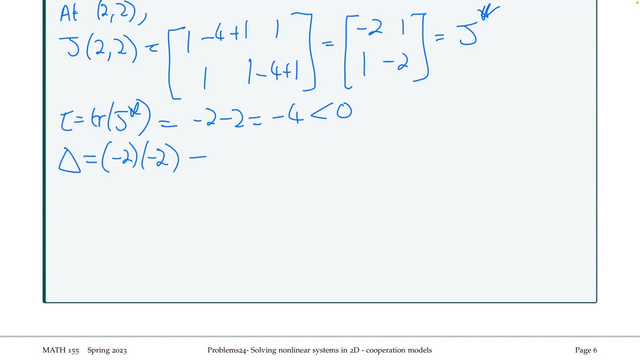 So here our trace is going to be minus 2 minus 2, which is minus 4.. Our determinant is going to be minus 2 times by minus 2,, minus 1 times by 1, 4, minus 1, 2 to 3.. 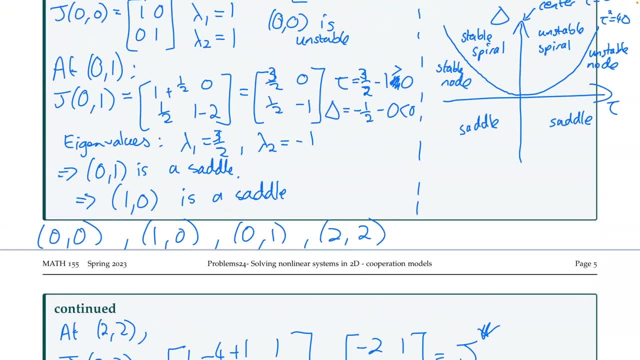 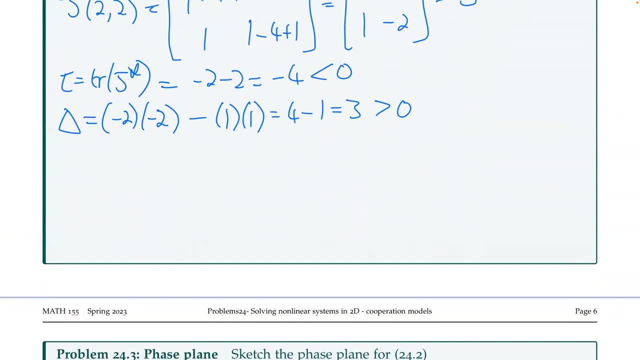 So you have a negative trace and a positive trace. So you have a negative trace and a positive trace. So that tells me, I'm somewhere up here. So that tells me, I'm somewhere up here. So that tells me, I'm somewhere up here. 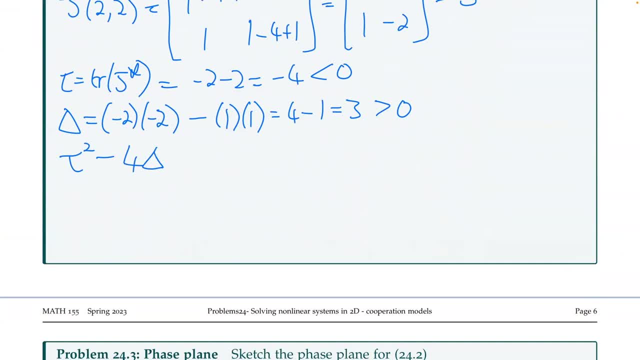 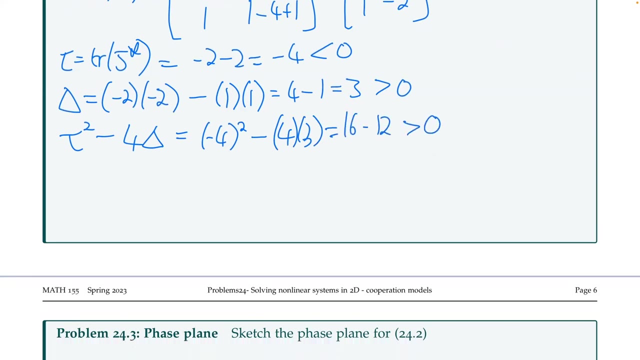 Trace squared minus 4 times the determinant. Trace squared minus 4 times the determinant, It's going to be minus 4 squared minus 4 times by 3, 16 minus 12,, which is positive. So we have real eigenvalues. 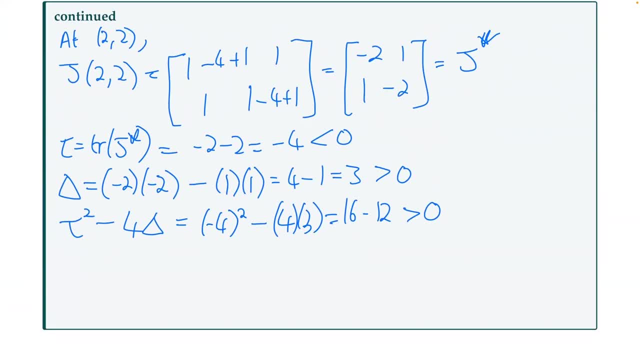 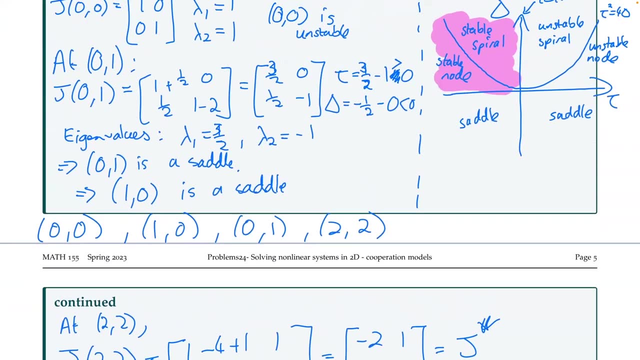 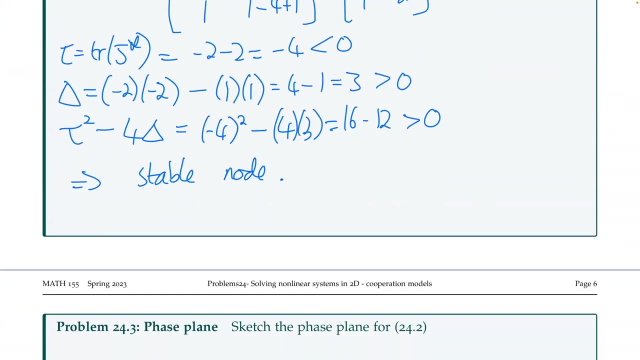 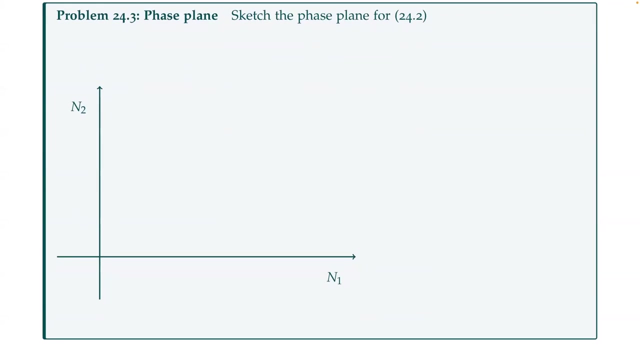 ε With a negative trace. So we have a stable node. Let's see what's going on in this region. Okay, From here, nonlinear systems will appear on the final Okay. So let's think about our phase plane. now I'm going to work through this one with you guys. 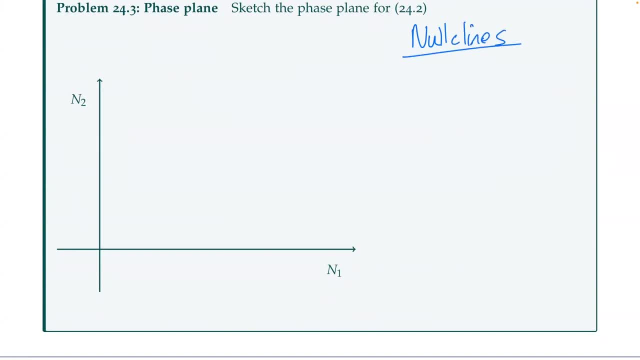 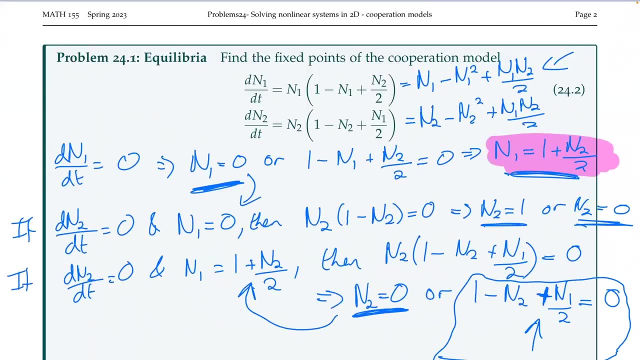 So whenever we're working out our phase planes, we need to think about our null clients. But if we've already worked out what our equilibria are, we've already found our null clients. okay, Because we have these conditions for when either of 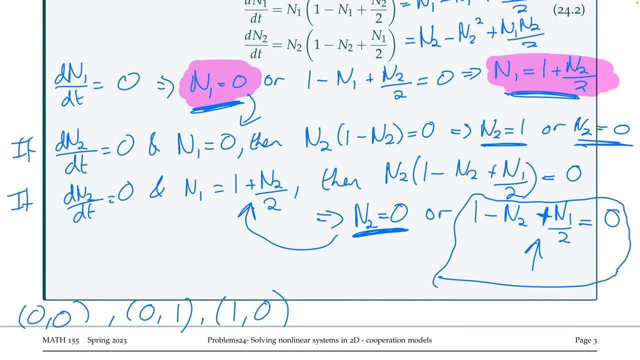 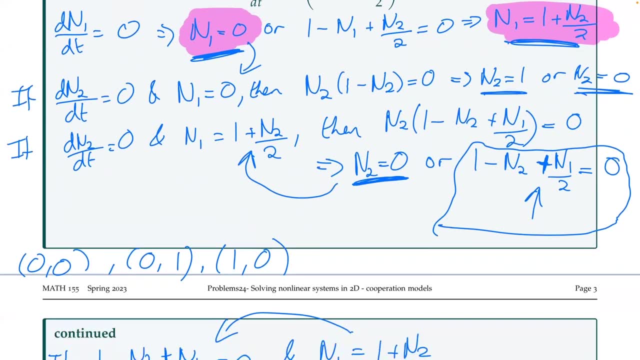 our equations dn1, dt or dn2, dt are equal to zero. So we know that n1 is equal to zero as a null client. Also, n1 is equal to one plus n2 over two is also a null client. We also know that n2 is equal to zero as a null client. 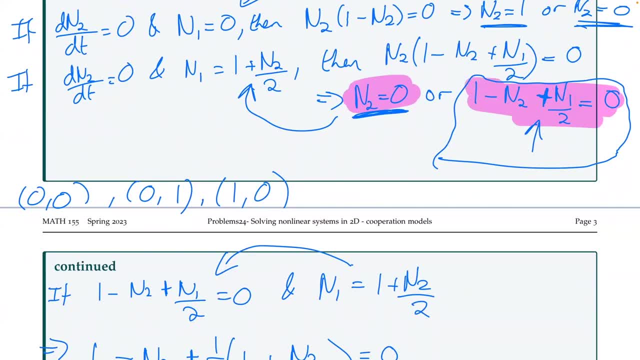 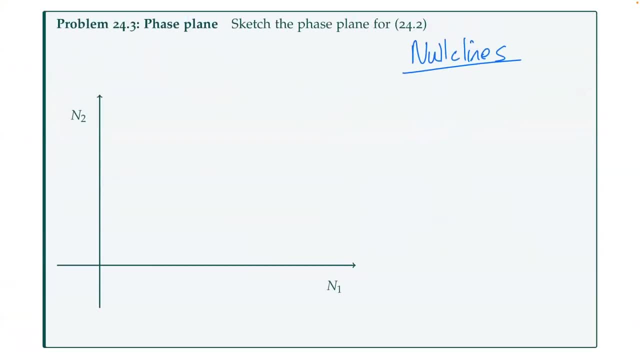 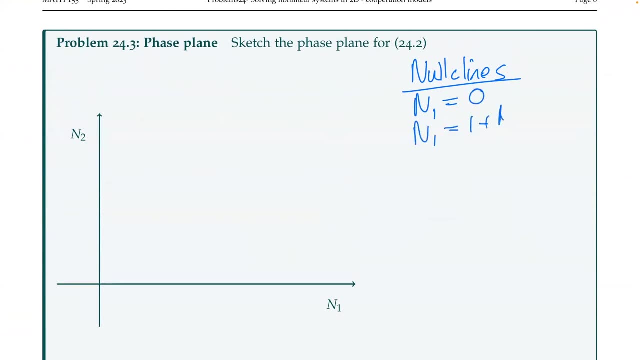 or this equation here on the right-hand side, will also give us a null client. So we already have our null clients. So they are: n1 is equal to zero and we've got. n1 is equal to one plus n2 over two. 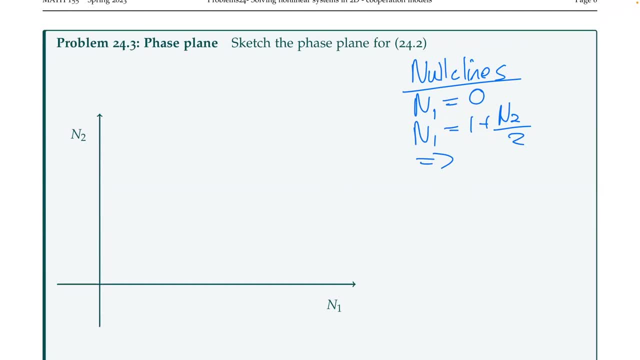 I generally, when I'm writing my null clients, try and rearrange them in terms of whatever is on the vertical axis. A few people asked me this at the office hours the other day and a lot of people got into issues with the gradient of their null clients. okay, 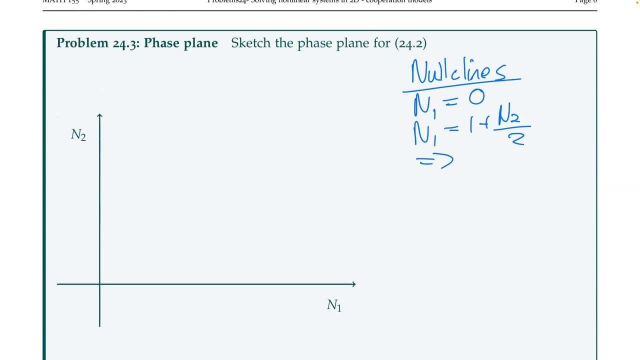 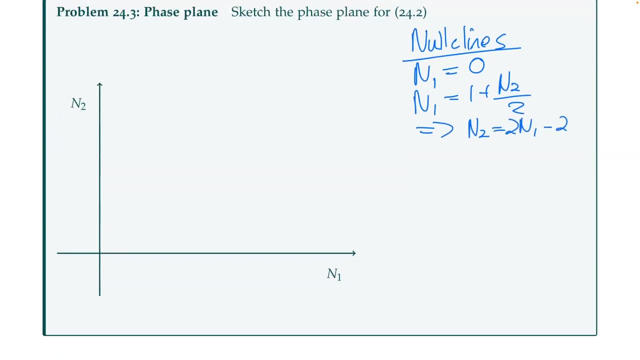 Rewrite these things in terms of what you can, in terms of what is on the vertical axis. So in this case I'm going to write it in terms of n2, which is equal to two, n1 minus two. My other null clients are: n2 is equal to zero. 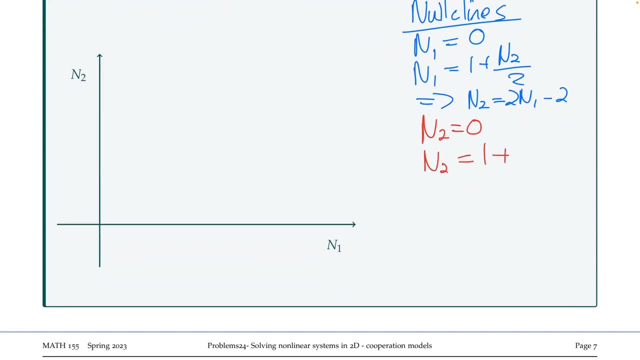 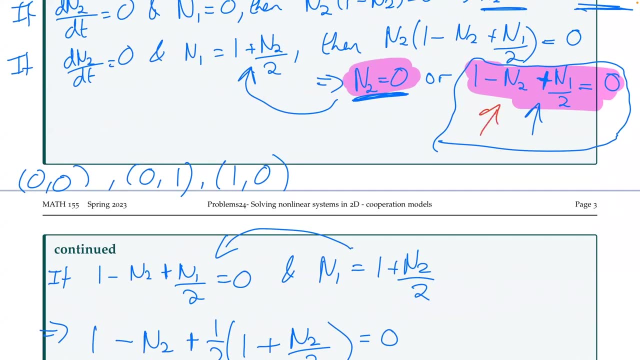 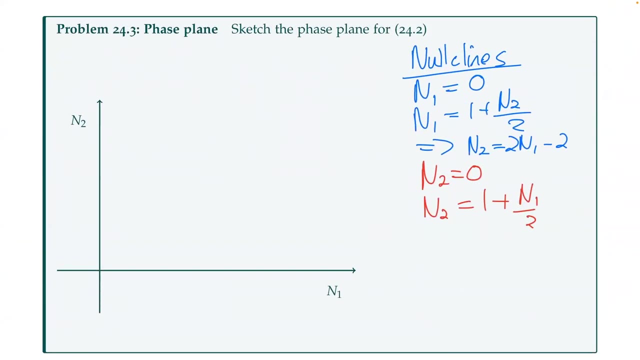 and similarly I can write: n2 is equal to one plus n1 over two by rearranging this thing here, So just adding n2 to the other side. Okay, so these are my null clients, So I can sketch them on. In population models you typically have null clients. 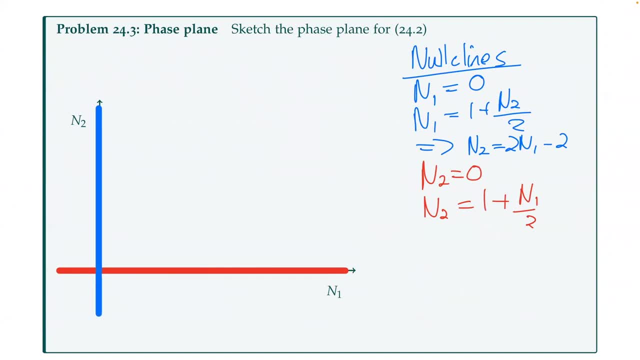 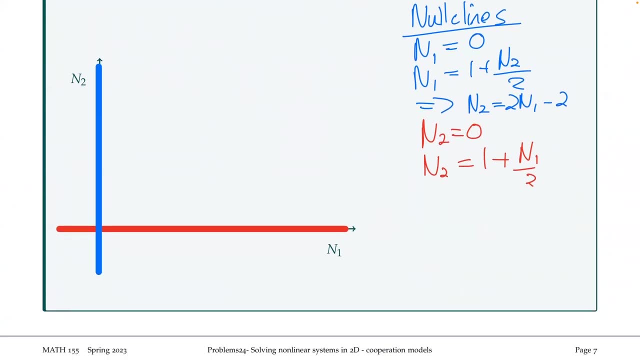 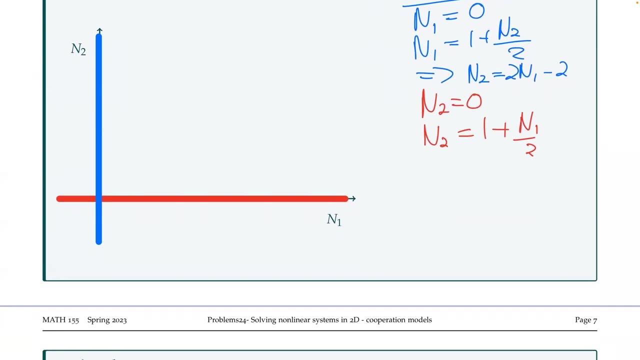 on the axes, so they're nice and easy to draw. We have this: we have two non-zero or two ones that aren't parallel to the axes. So the line n2 is equal to two, n1 minus two. this is where that is equal to zero. 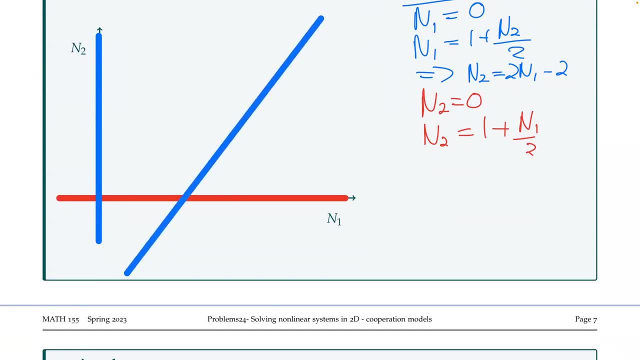 For the promote n2, we can just copy and paste it into that N2 line. We can do that. So we know that that will go through one zero down there, point one zero. We know that because we know that we have an ребrea. 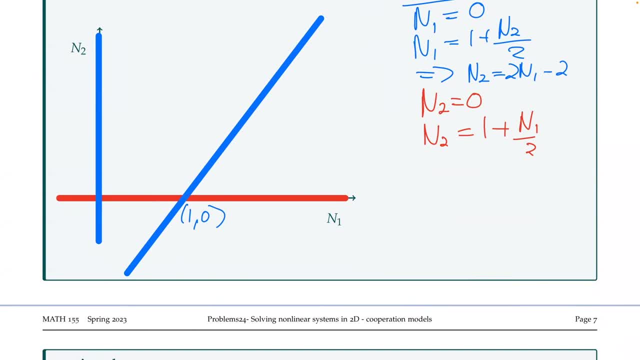 on the axis. when n1 is equal to one, What else do we have? We have: n2 is equal to one plus n1 over 2.. be a half and the intercepts are equal to one. we draw that So it looks something like that. 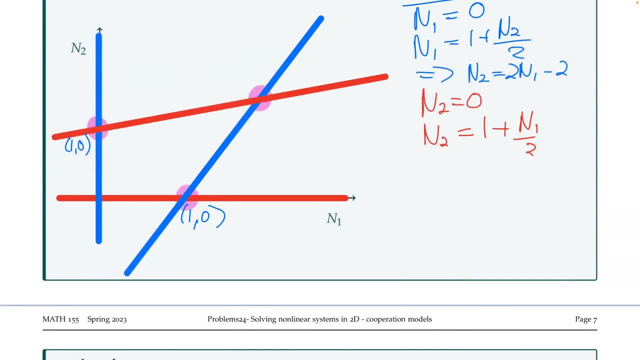 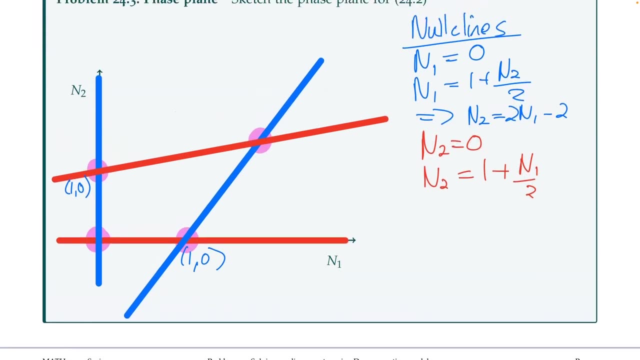 So we have equilibrium whenever we have an intersection between a blue and a red line. here Some tips on drawing phase planes. whenever you're drawing them, whether it's for a homework assignment or it's an exam- I've said this before- please make them big so it's easy to. 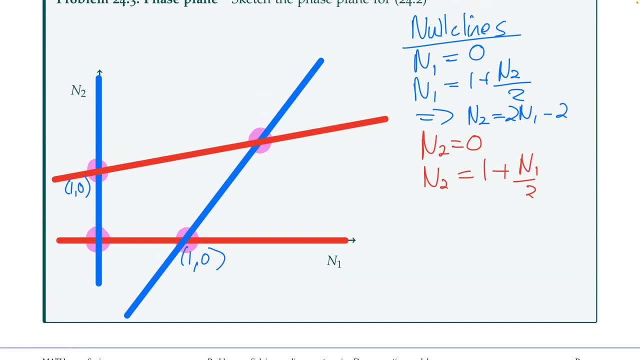 see what is going on. give yourself room to draw on everything, Please. also, you don't have to do this, but you need to label it somehow. So sorry, you don't have to color code it, but you need to label it somehow. If I've drawn these all as black lines, I need to say that this is say. 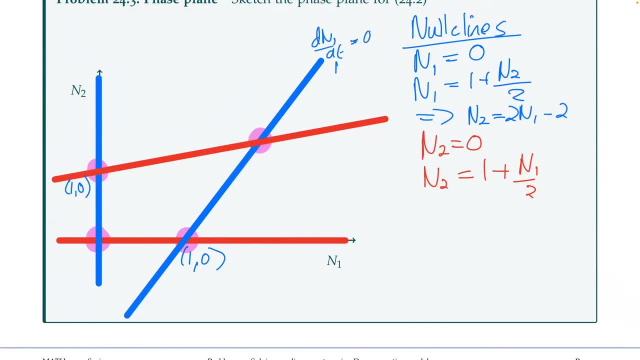 the line that I'm drawing. So I'm going to say, I'm going to say, I'm going to say, I'm going to line dn1. dt is equal to zero, And this is the line. n2 is equal to 2n1 minus two. Okay, You need. 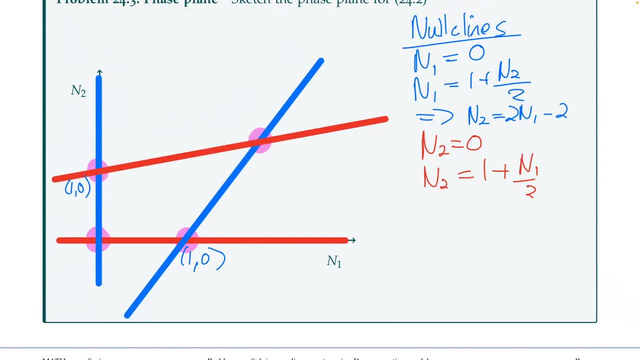 to provide some sort of key to what is going on here. I like to color code it because it looks neat. Remember what are the null clients for my n1 variable and what are the null clients for my n2 variable. You could dash them. That's another way of doing it: Solid and dashed lines. it's. 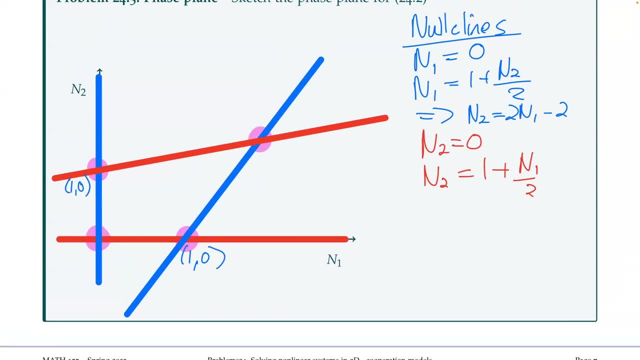 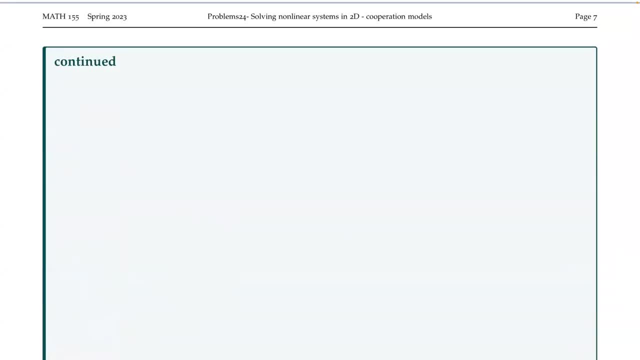 fine, Just make it clear What is going on by having a key of some kind. Okay, So I've got my core equilibrium here. What do we know about? we don't know our direction field, so let's work that out. 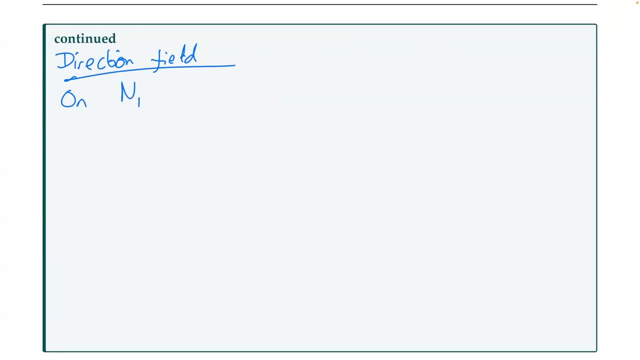 So here I'm going to focus on what's going on in the axes On. n1 is equal to zero. We know by definition that dn1 dt is equal to zero. What is going on with the dn2 dt? So typically as well? at this point I like to draw on 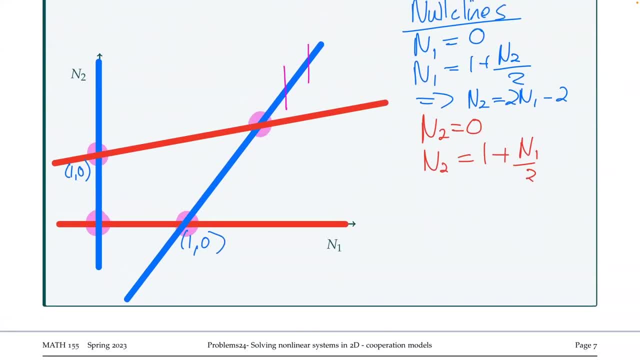 some horizontal and vertical lines. So I know my blue null client but I must be moving up and down. I can't be moving left and right. And we know my red light null client must be moving left or right. I can't be moving left and right. 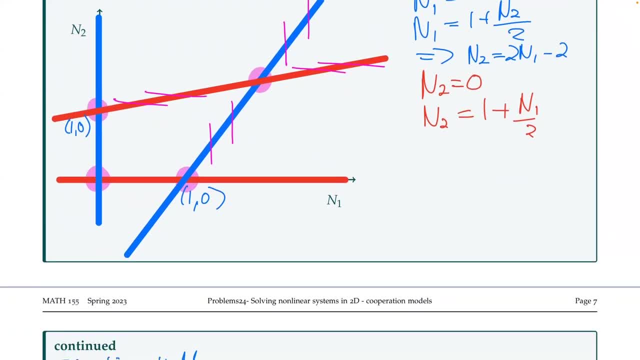 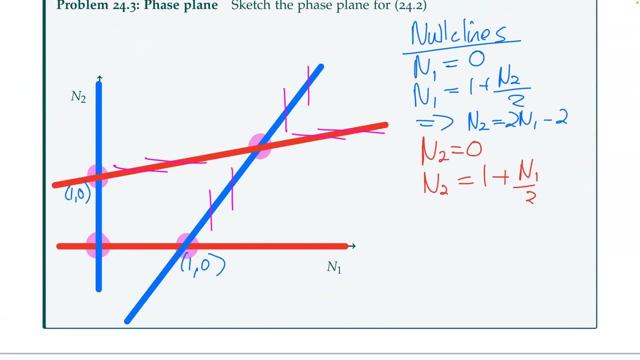 up or down. that helps me make sure i don't accidentally put my arrows on the wrong axis. so when, whenever we're doing this direction field, we're looking, say, on our null clients, we're actually going to be looking at m1 is equal to zero, so we're going to be looking at this one. 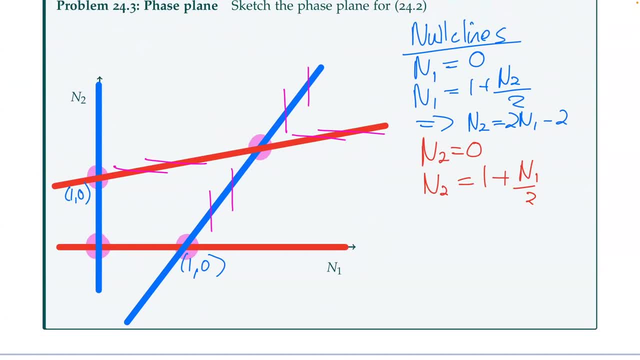 and this one first. what we're doing is we're saying, okay, i'm stood at say a point on this, no incline here. i know that i can't be moving left or right because dm1- dt is equal to zero, and i want to know: am i moving up or down? likewise, what happens if i go through an equilibrium? 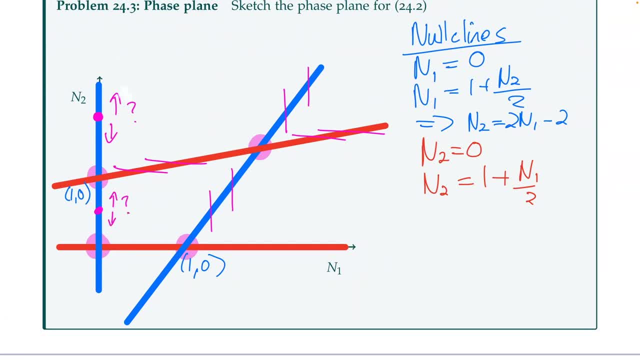 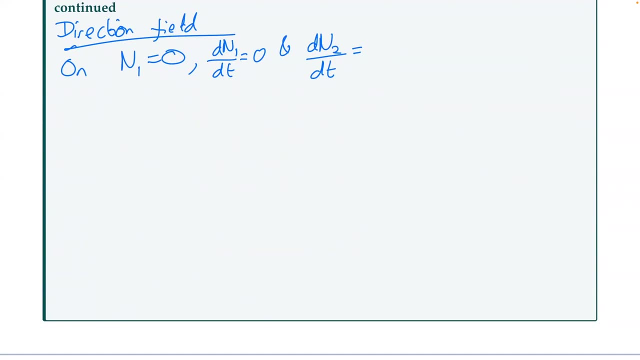 down here. am i moving up or down? okay, so i'm stood on this line. n1 is equal to zero. i know i can't be moving left or right. i want to know: am i moving up or down? so all i do is i substitute this equation here, whatever it is into this equation, for dn2 dt. so we know dn2 dt. 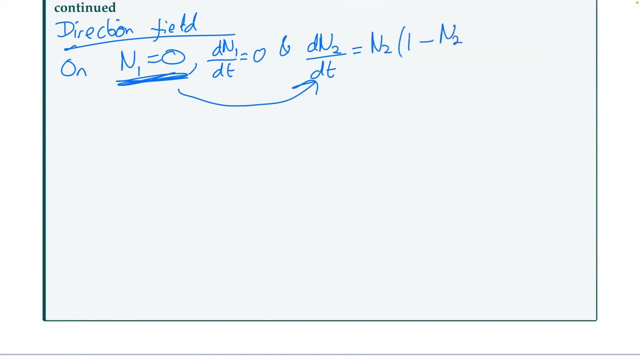 is equal to n2 times by 1 minus n2 plus n1 over 2.. now here you might have an equation for n1 and n2 that you're substituting in and you here you'll be eliminating one of these variables. in this case there's just an n1. we know n1 is equal to zero, so we can eliminate. 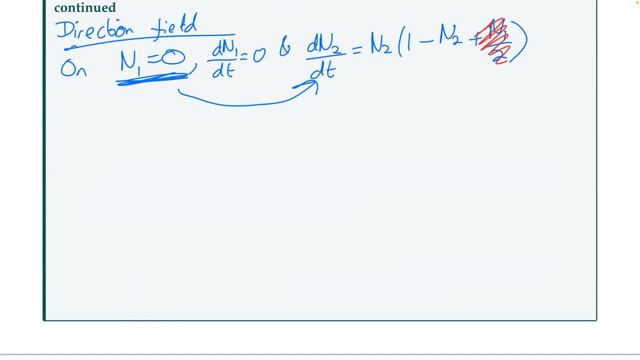 this n1 here. so we have dn2 dt is equal to n2 plus by 1 minus n2, and what we care about is when is dn2 dt positive and when is it negative, depending on the variables on the right hand side. so what can we say? well, dn2 dt is going to be positive. 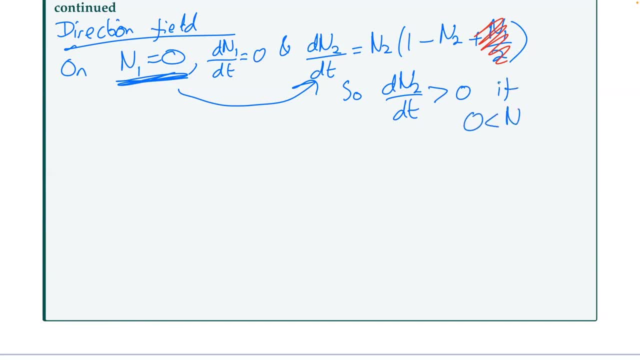 if n2 is positive and it's less than 1.. this will give us arrows moving up and it's going to be negative. well, it's going to be negative if n2 is negative but we've got population sizes. we can't have population sizes. we don't care about what's going on if n2 is negative. but if n2 is greater than one, 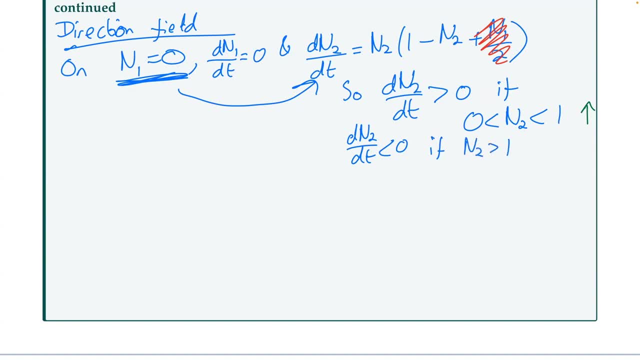 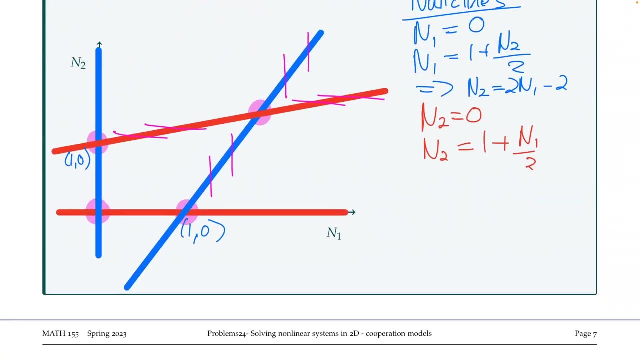 1, then dn2 dt is going to be negative. So let's go back up to this diagram here. That means if we are, if n2 is greater than 1 and we're on this line and 1 is equal to 0,. 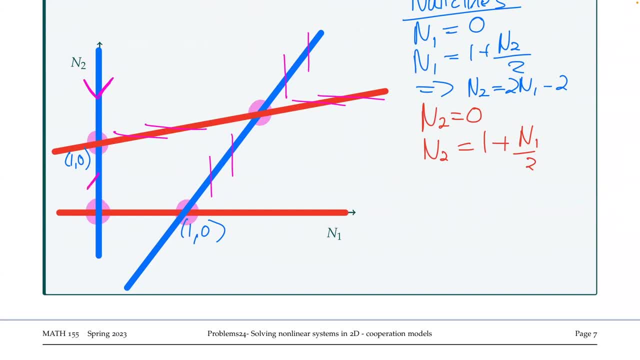 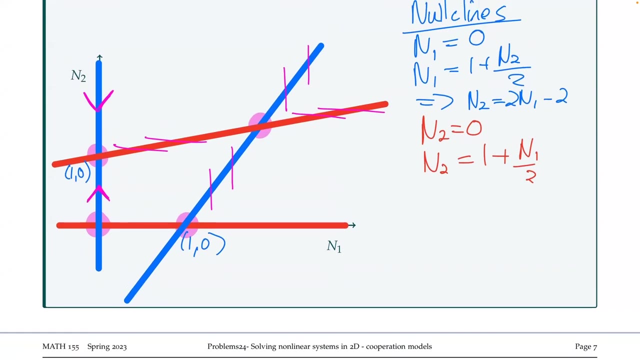 we must be moving down, And if we're between 0 and 1, we're going to be moving up. Now you can work through the second one as well in your own time if you want to, Because this is symmetric. I know it's going to be exactly. 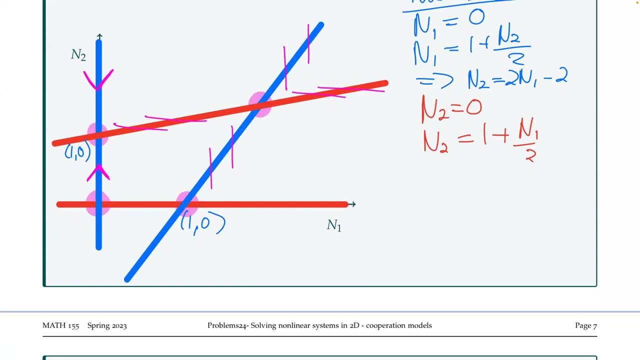 the same on the other side. If I flipped all my n1s and n2s around, nothing changes, okay? So in this particular case, I know that this is going to be an arrow going this way and this is an arrow going this way. 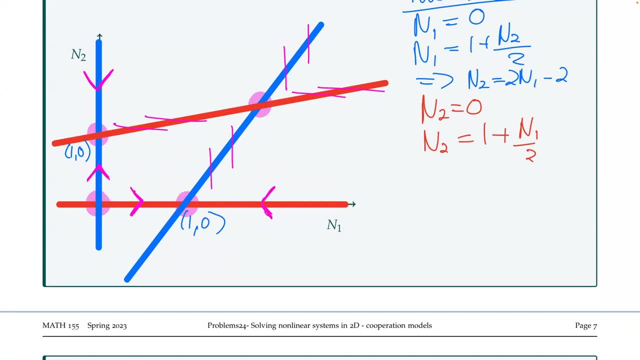 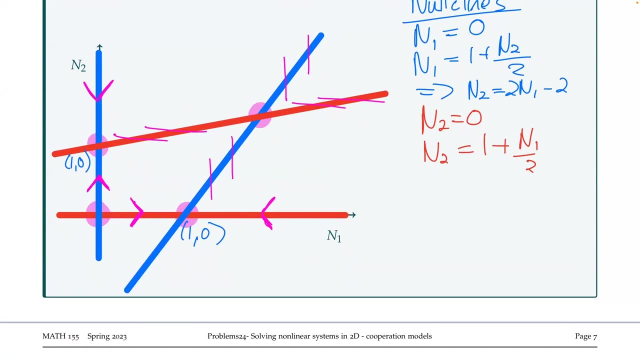 This is because the system is perfectly symmetrical. Okay, Another little trick we can do at this point is, if we know what's going on on these null finds here, we change direction as we go through this point. okay, That means imagine if I, if I zoom in. 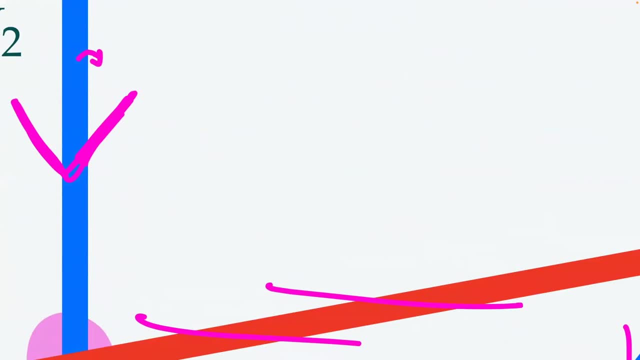 here, and I step a tiny little bit off this axis here. I'm still going to be moving, mostly down. I'll also, if you move, be moving a little bit left or right because we're no longer on a null client, but i'm not moving up. 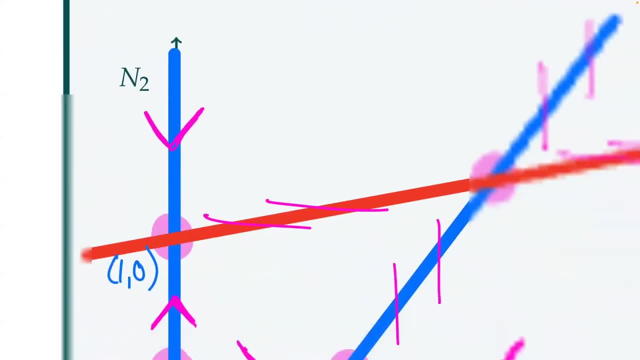 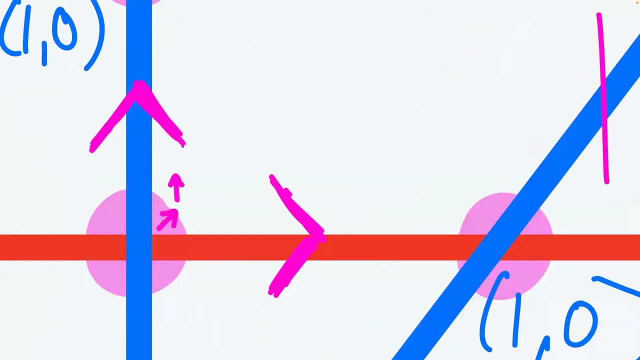 i know i'm going to be moving down in some direction. likewise here, if i step a little bit away from the origin here. i know i have to be moving up, but i also have to be moving to the right, okay, so in this case i don't actually have to worry about working out. what am i, uh, what my? 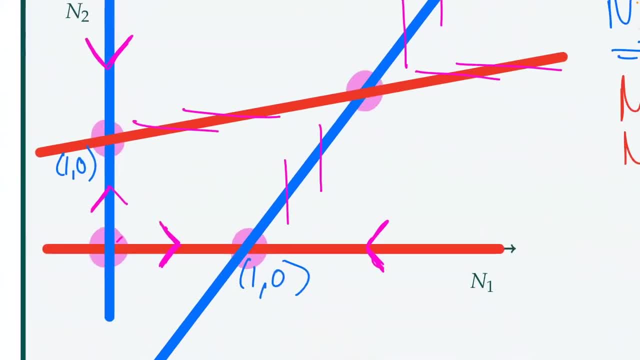 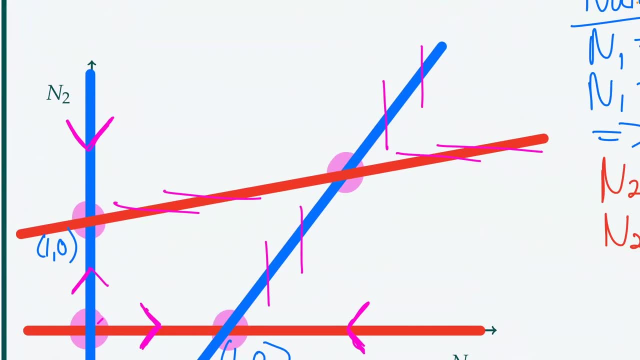 arrows are doing on these null clients working out the individual direction field, because these are continuous functions. if you move a little bit you're not suddenly going to change direction, unless you go through an avalybrium. so that means i know in this region here. well, actually, let's. 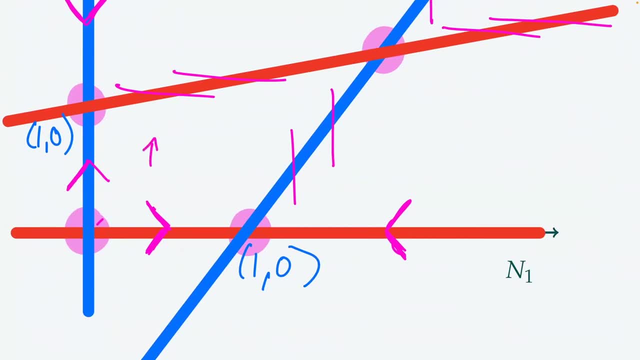 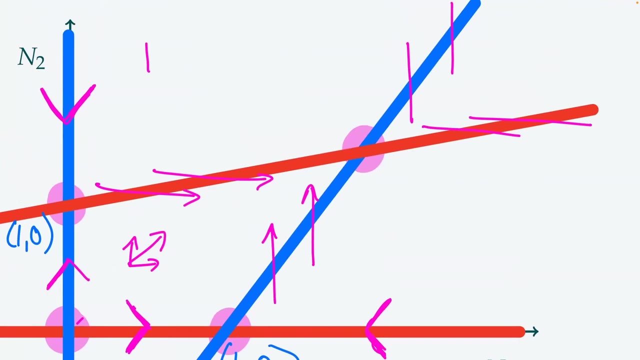 start in this region, because this region is going to be the easiest. i have to be going up and to the right. okay, so that tells me that these arrows here must be going to the right and these ones also have to be going up in this region, here at the top. i know i'm moving down because i'm moving. 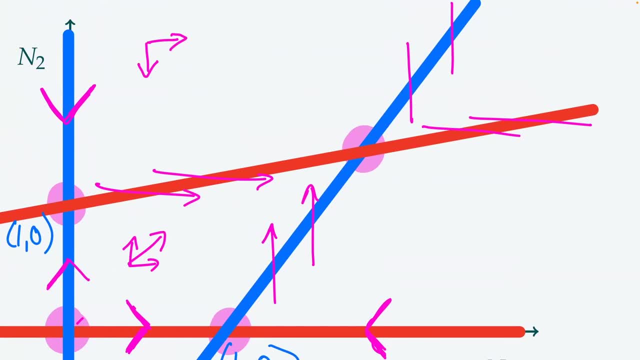 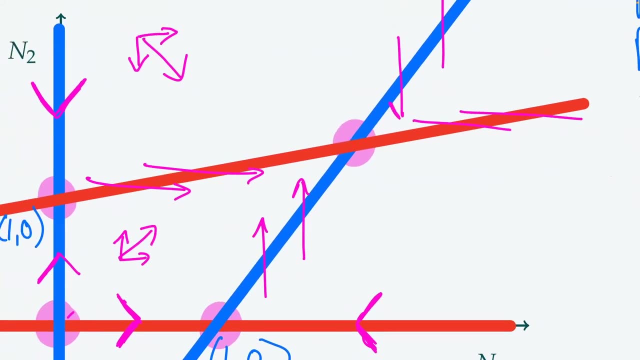 down. i'm moving up because i'm moving lower. i now always have to do less than i can down on the axis and I have these red arrows moving to the right. so I know I'm moving down into the right, so I'm moving in somewhere in this direction. Otherwise these arrows up here must be down. 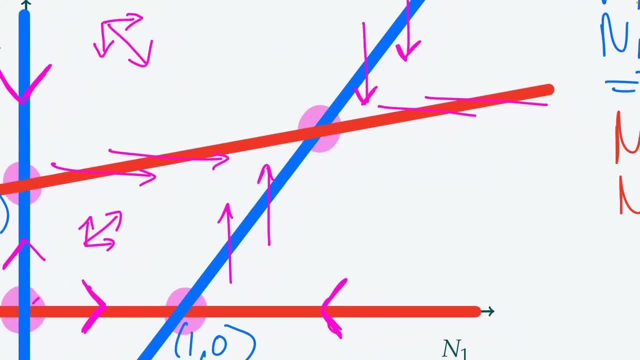 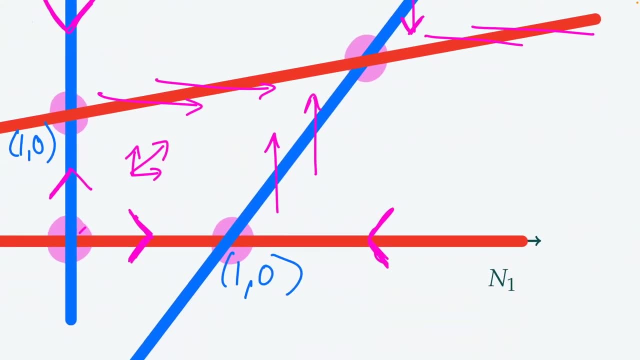 because the ones on the axis are down. So over in this, let's do this bottom right quadrant. here I know I have to be moving to the left and I'm also moving up because of these arrows here and here It's actually moving in this direction. That leaves me one more quadrant here. 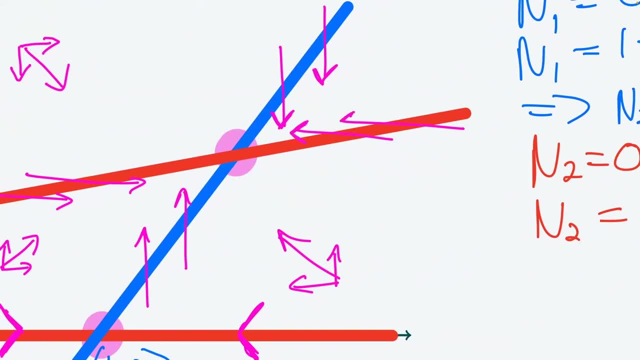 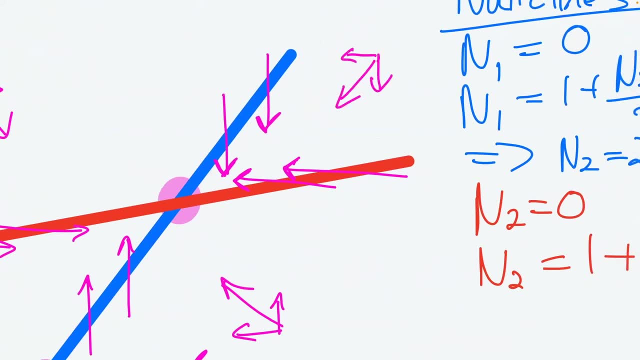 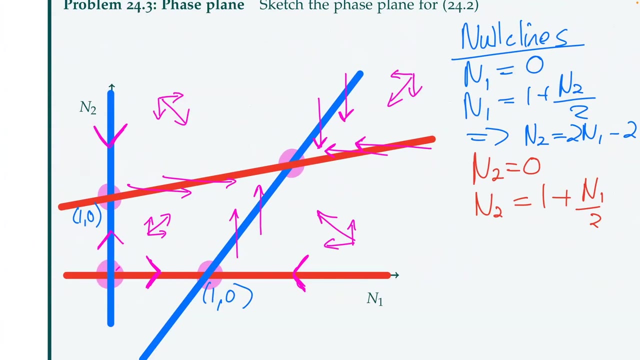 because I'm moving to the left below, I must still be moving to the left because I've not gone through a fixed point here. So in this region up here I know I must be moving down and to the left. So you don't necessarily have to work through every single combination of things. 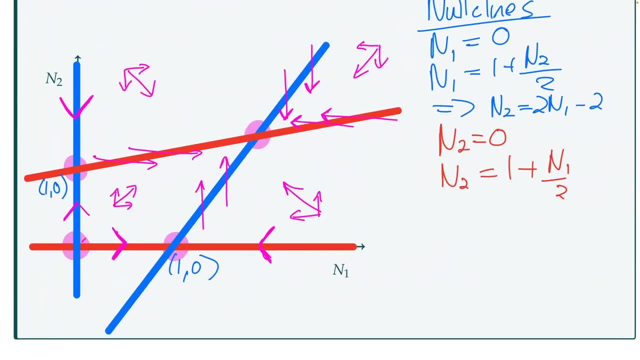 on the axis, but you do have to work through every single combination of things on the axis On your null clients. I didn't have to actually work out what all of these arrows were on my non-zero null clients. I could just do it by deduction. 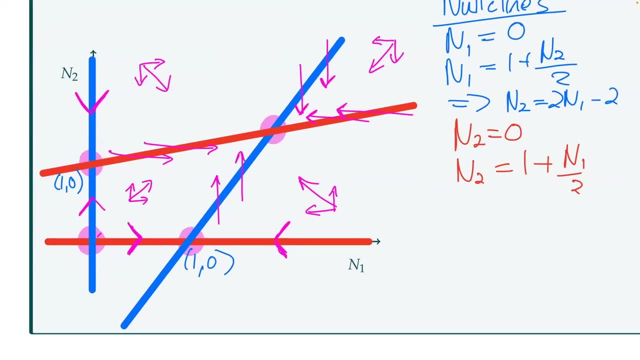 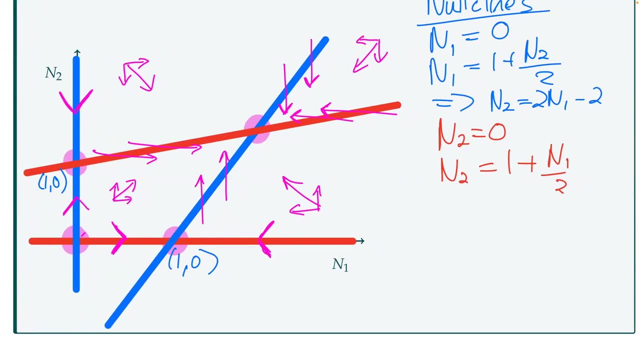 So if this was in an exam, I would allow it, as long as you get the right answer. The only problem with doing this is that you don't leave any of your workings there. I have workings here for this one null client, and then I basically deduced everything else. 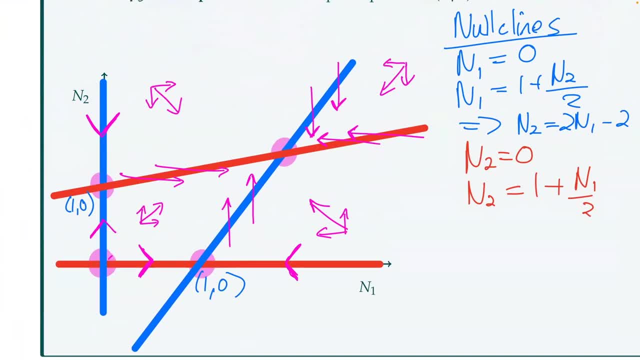 That is a little bit of a risky thing to do. I would give full marks for this if you got it correct. But just be aware that if you do that process of deduction you are leaving yourself a little bit open because you haven't shown any workings. 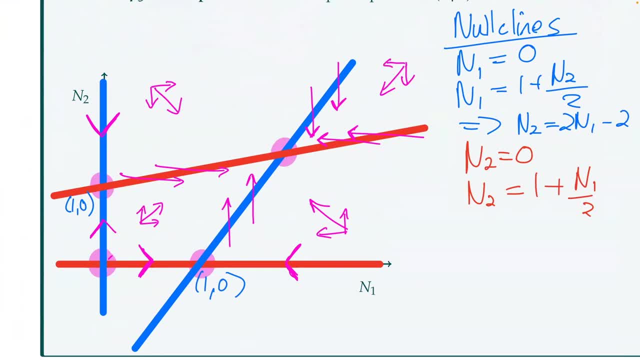 So it is correct, and I will give a few full marks for this, but just be aware of the consequences of doing that. Of course, you can always check these by substituting them. So if we draw some trajectories here, you see that if we started at non-zero value for n1 And n2, we 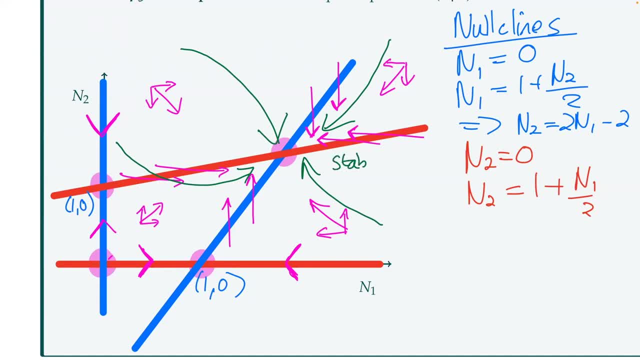 tend towards this equal line on this distance here as well. So that's a better way to keep this coexistence equilibrium here. We'd already worked out that this was a stable node, but we can see it from our phase plane as well, And this was the point two, two. 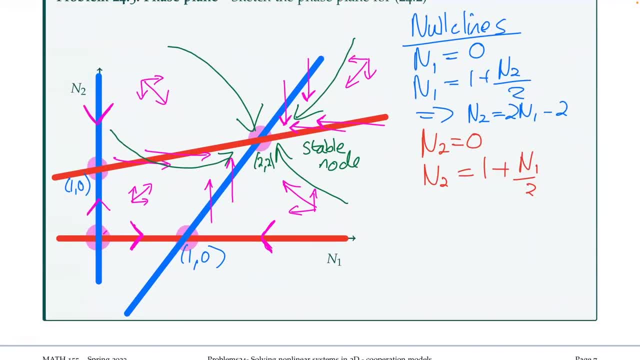 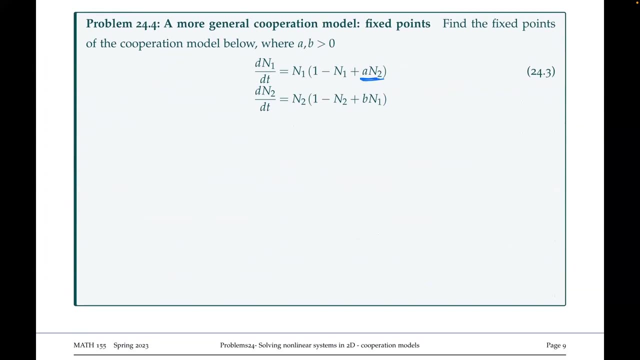 Okay, any questions? Okay, for the last few minutes I'm just gonna go through a general version of this model. Okay, so before we had A was equal to a half and B was equal to a half, but we could just think about a general form of this model. 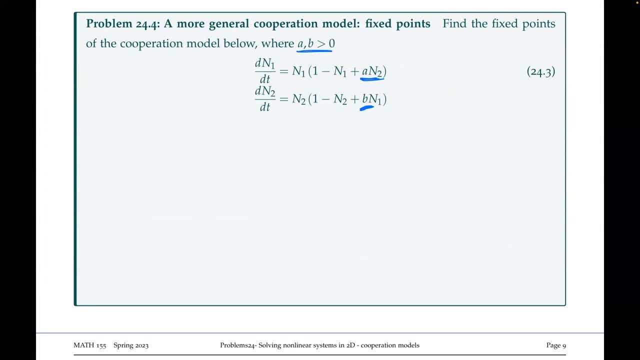 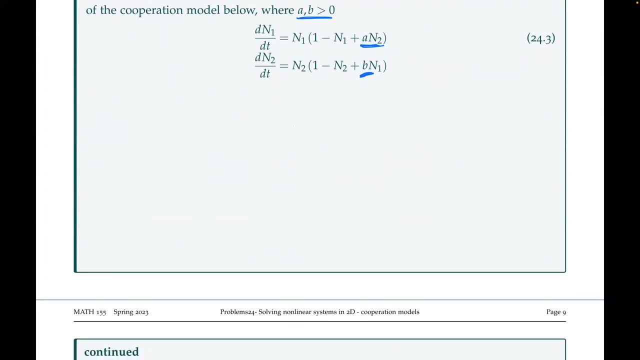 where we have parameters, positive parameters A and B. So we don't know what these are and we can work out what goes on in this case. So I'll leave working out the fixed points as an exercise I've mentioned. we can turn this into a linear system. 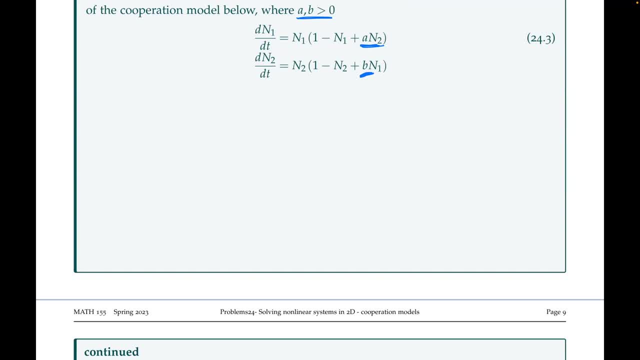 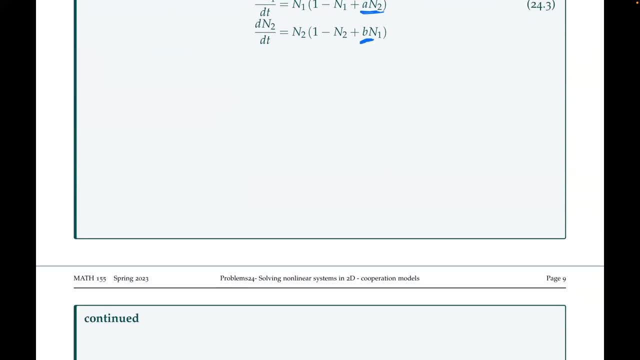 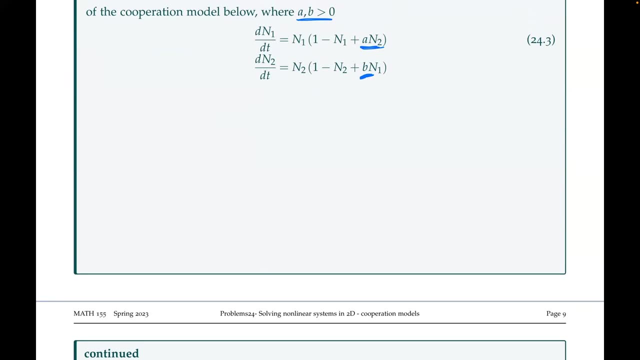 to work out our fixed points. So for our coexistence equilibrium, it turns out that if it exists, we have- Sorry, my pens have died, There we go. If it exists, we have N1, N2 is equal to one plus A. 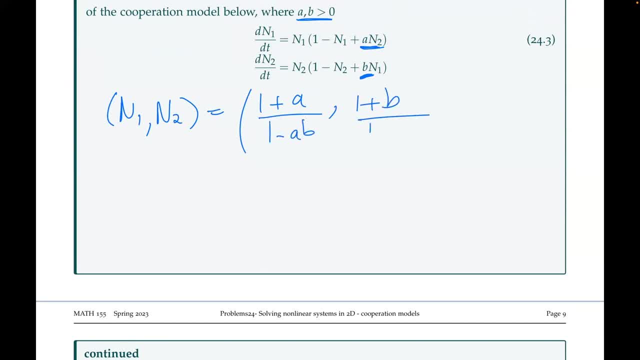 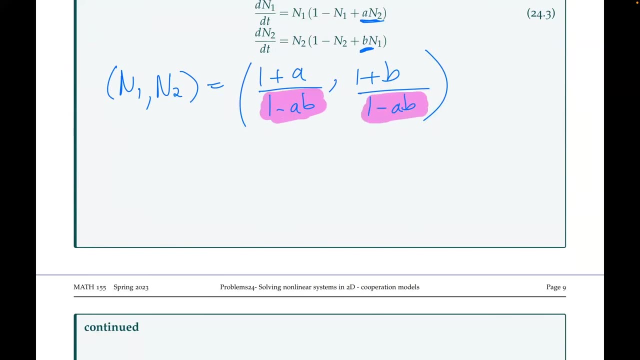 one plus B and both of these over one minus AB. Okay, So there's the answer. and try and work towards that if you can during time. Crucially, this is only gonna be biologically realistic. The numerators are always positive. 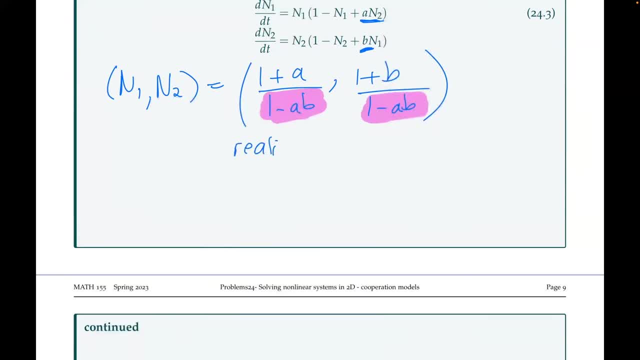 The denominators are only positive if A times by B is less than one. So this coexistence equilibrium, for instance, is positive. So we can think about two possibilities. Now we can think about the possibility of what happens if AB is less than one. 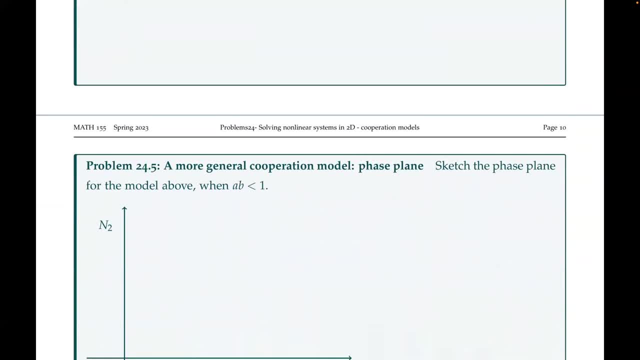 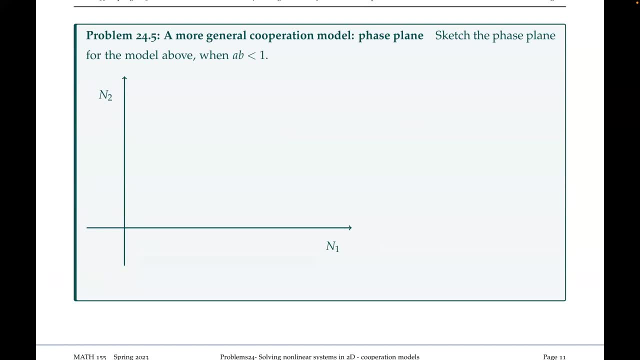 What's our face grain gonna look like? So you can have a go at sketching this. We've actually already got this case up here, because our A was equal to a half and our B was equal to a half In the example we've just been through. 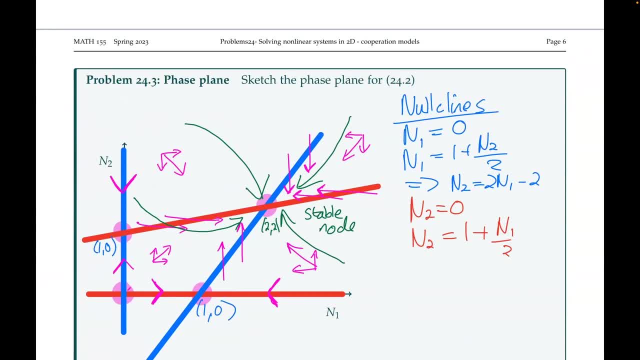 AB was less than one and then the last one was just less than one. So we can have a go at sketching this. We've actually already got this case up here, Because our A was equal to a half and our B was equal to a half. 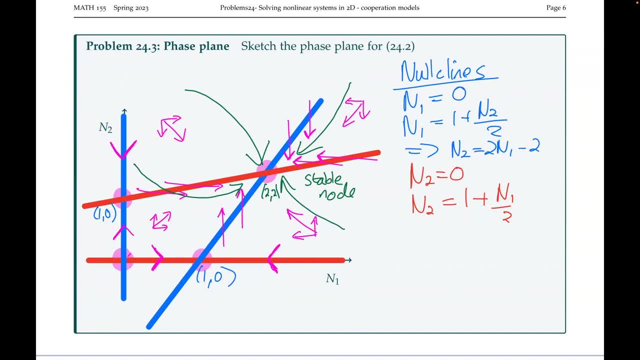 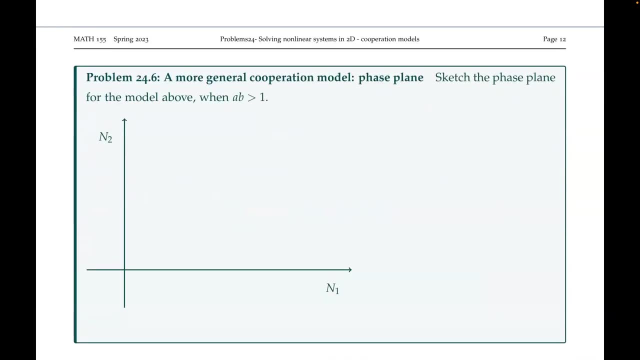 AB was less than one, so our phase plane ends up basically looking like this: okay, The location of that fixed point will vary as A and B varies, but qualitatively it looks like this. Again, you can have a go at sketching the general form. Let's think about the other example here. 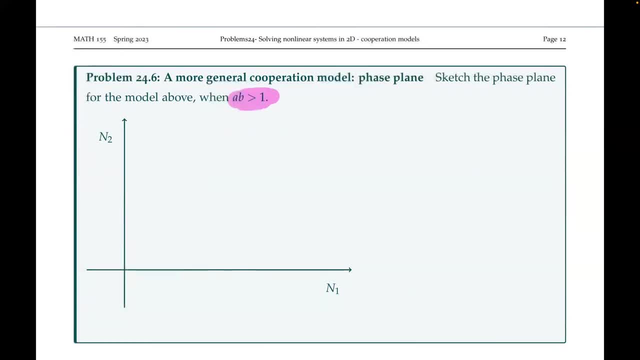 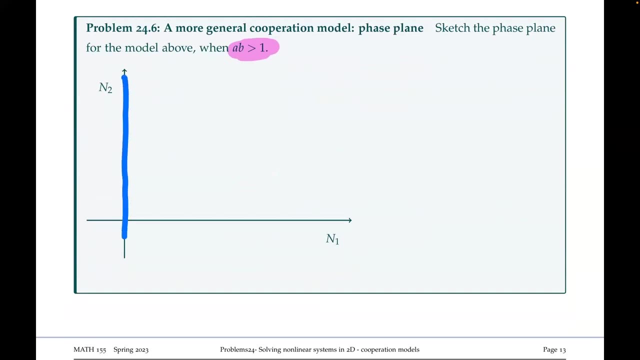 AB is greater than one. So if AB is greater than one, we have no coexistence equilibrium. So what does that mean? Well, let's draw on our nullplanes that we know about. We know that we're always going to have one here on my N2 axis and have one here on my N1 axis. 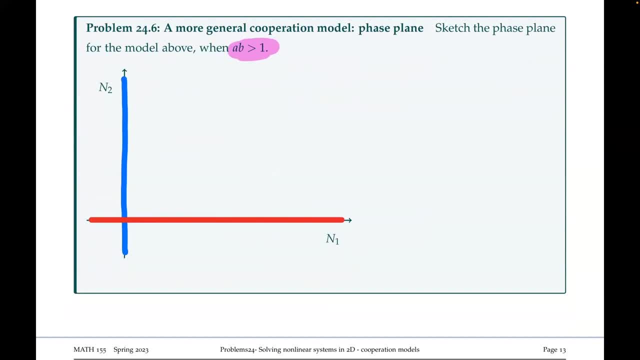 that we had previously. We know that we don't have a coexistence equilibrium, so that means that the nullplanes can't intersect. I see you dividing the C's there. That's basically what's going on here. okay, They can't intersect, They can't intersect, They can't intersect, They can't. 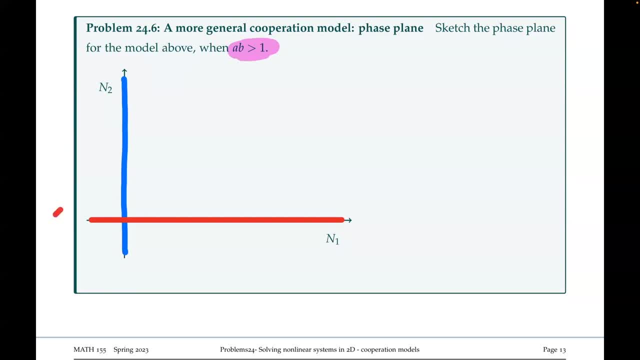 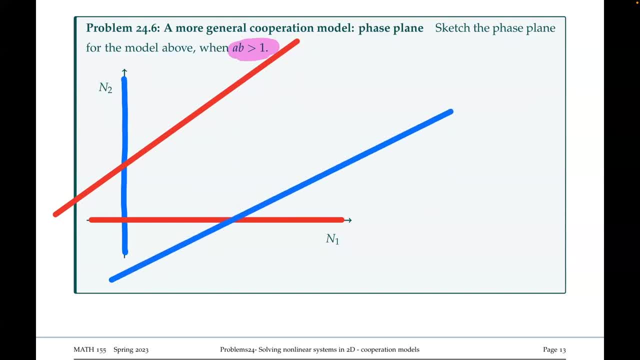 and this one. I have to go like this. What it means is these lines are diverging. They never intersect in this positive quadrant. If they intersected, you'd have something right over here. These lines would have to intersect somewhere, right? So if they intersect, then we have a. 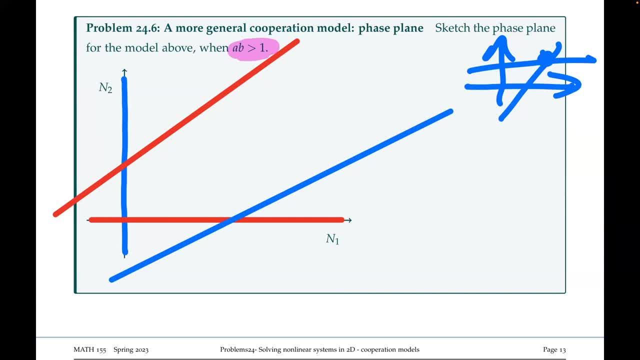 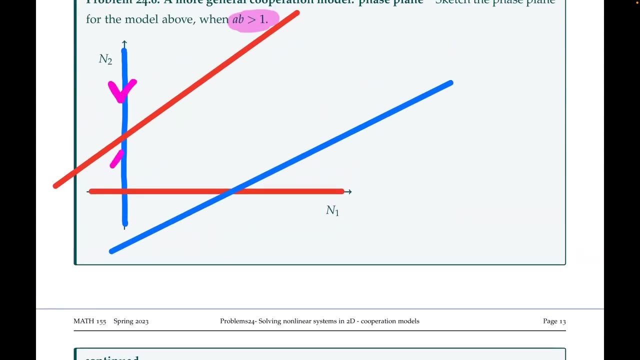 coexistence equilibrium. but we know that we don't have a coexistence equilibrium, so we know that my nullplanes have to look like this. We can also deduce what we had from our previous diagram. So on a previous diagram we had these arrows on our axes pointing in these directions here. 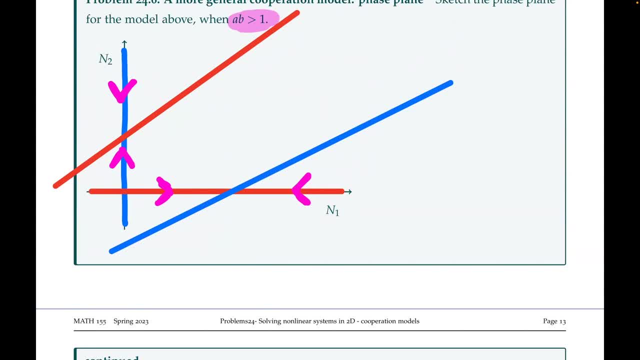 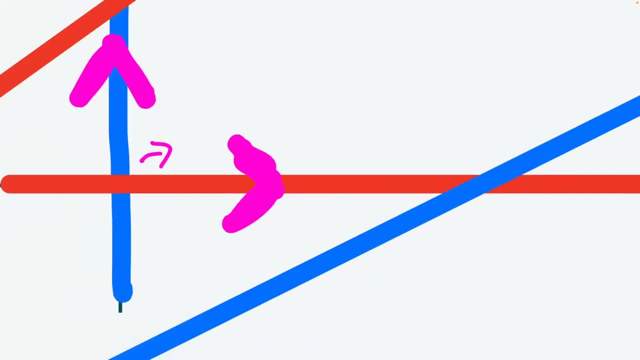 Just like I did on the previous diagram, I can think about what happens if I move a tiny bit away from the axis in any of these directions. I'm going to move a little bit away from the origin here. I know that I must be moving. 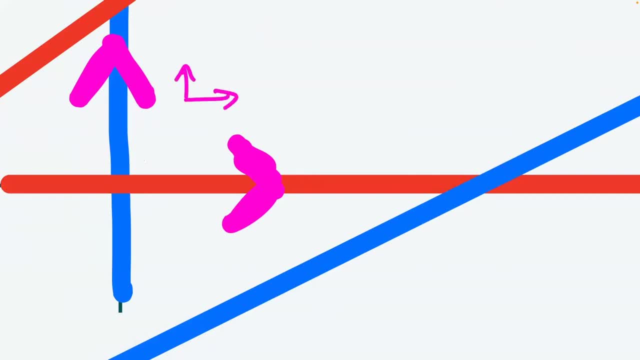 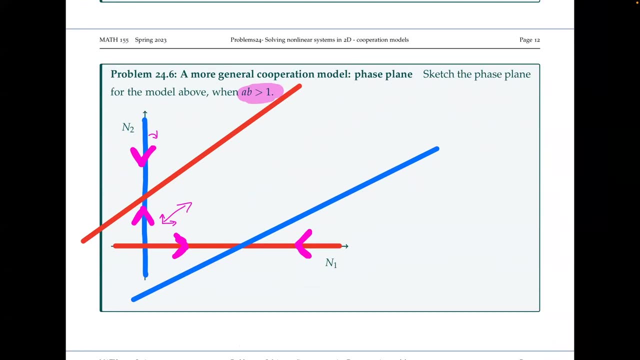 up and to the right, because that's what's going on on the axes. That means in this middle block, here I must be moving up and to the right, About in the top left, that little triangle above the red line. well, I know I still must be moving to the right. 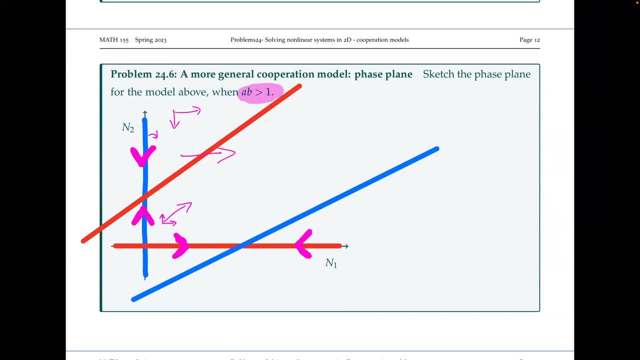 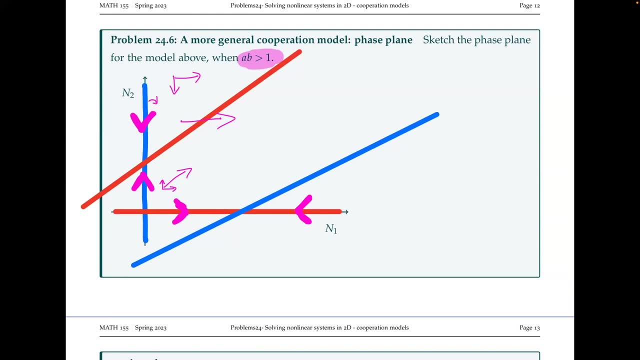 I'll also be moving down. So here, I know I'll be moving down, and to the right, In this bottom triangle below the blue line, I know I must be moving left, And because the arrow over here is moving up, this arrow has to be moving up. 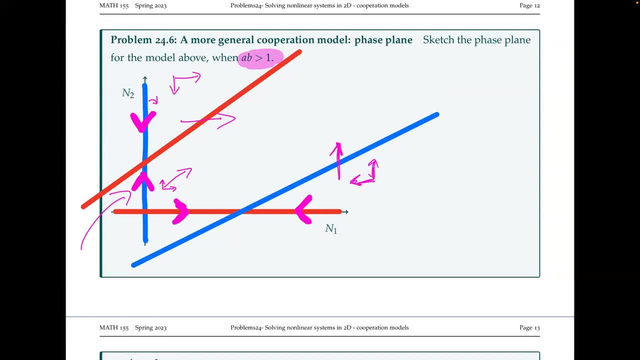 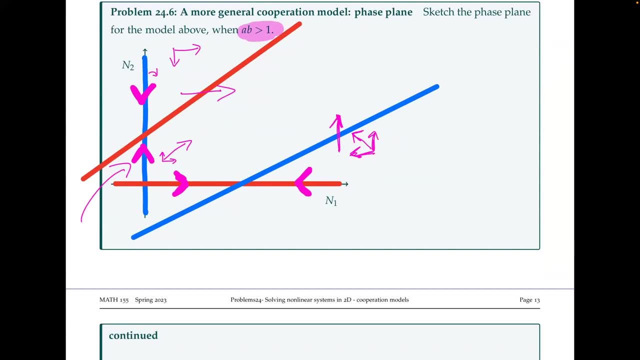 I'll be moving to the left. So in this region I'm moving up and to the left. That's all I need to tell me what's going on here. If I start at any non-zero values for n1 and n2, suppose I start over here. 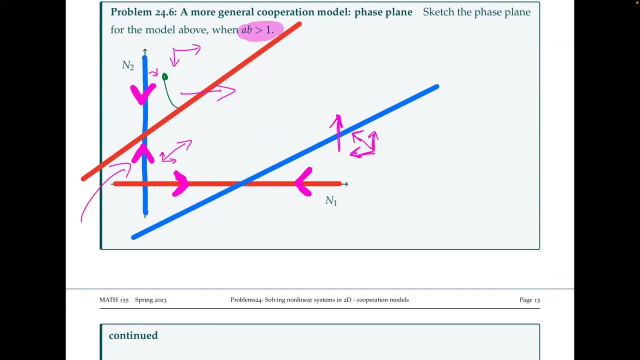 I'm going to start by moving down and to the left. I cross the nulled line horizontally going to the right, and then I'm moving up and to the right and I just keep going in that direction. Likewise here, I'm moving up and to the left. 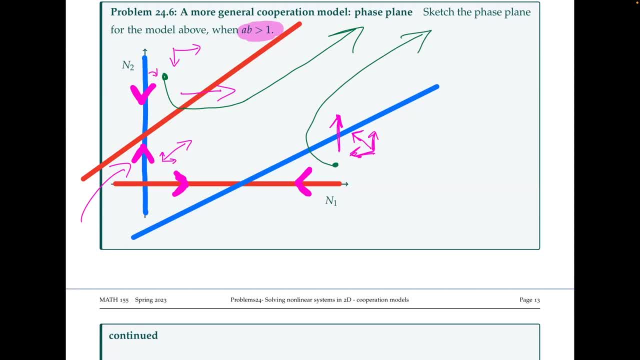 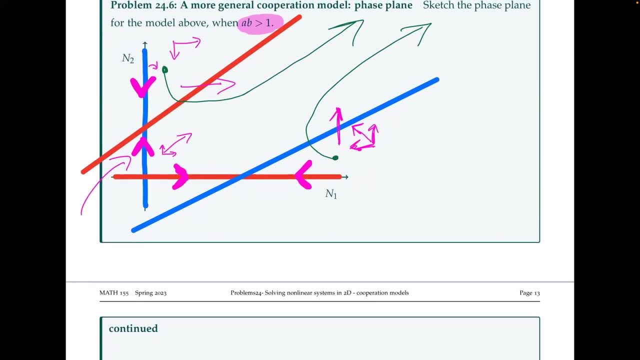 I keep going up to infinity. So what this means is that these populations- there's a positive feedback between them, and they keep growing and growing and growing and they go up to infinity, which isn't very realistic, But it means that there's a positive feedback between these populations. 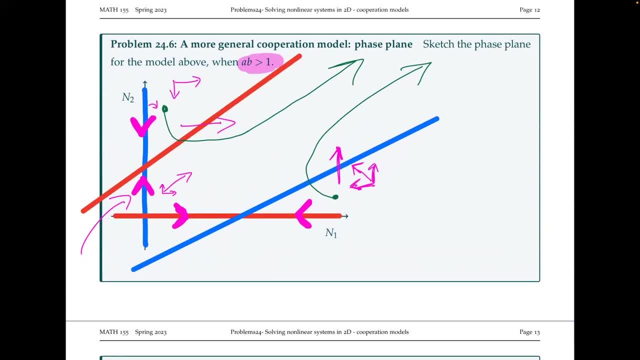 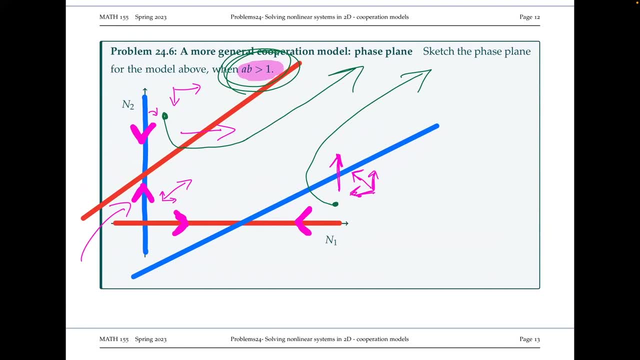 There's no coexistence equilibrium. everything just goes up to infinity. Okay, so this is saying something about what is the strength of this mutualism between these species. If it's stronger than the intraspecific effects, then everything blows up. Okay, I'll see you on Wednesday. Thank you. 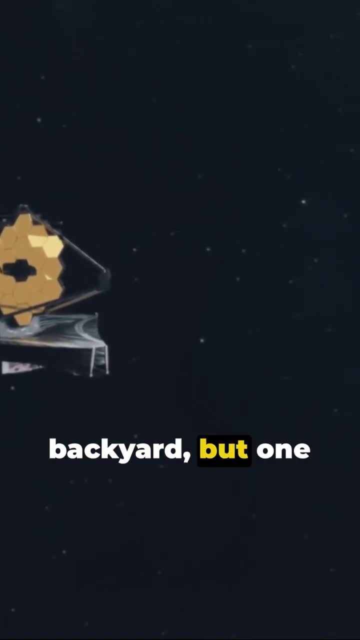 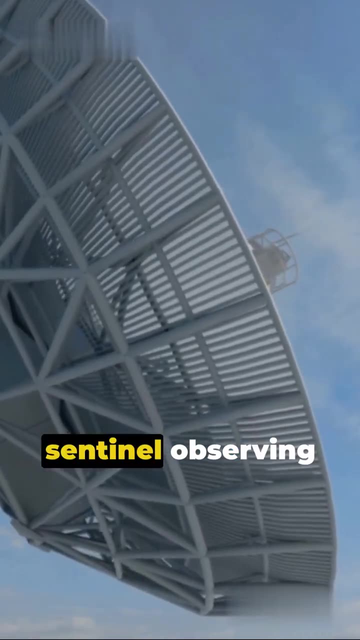 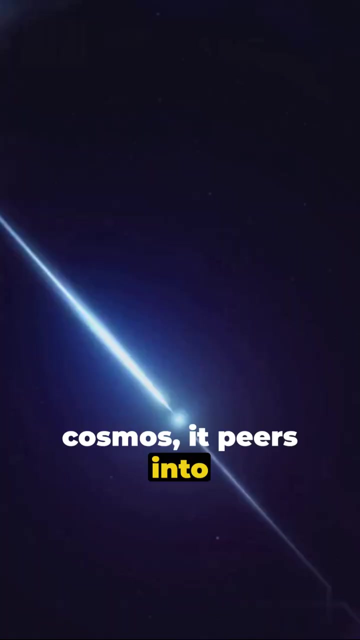 A picture, a telescope, not like the one in your backyard, but one situated in the vast expanse of space. This is the Fermi Gamma Ray Space Telescope, a silent sentinel observing the most energetic light in the universe, gamma rays Unveiling the mysteries of the cosmos it peers into the heart. 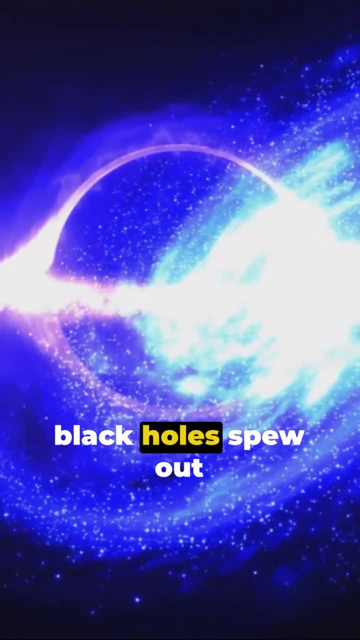 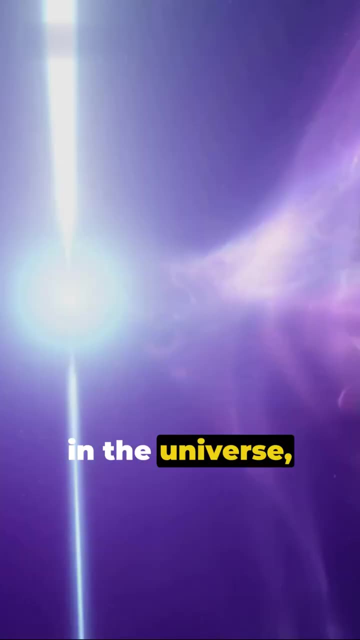 of active galactic nuclei, where supermassive black holes spew out high-energy jets. It's also on the lookout for gamma ray bursts, the most powerful explosions in the universe events- so intense they briefly outshine entire galaxies. For over a decade, the Fermi Telescope has been 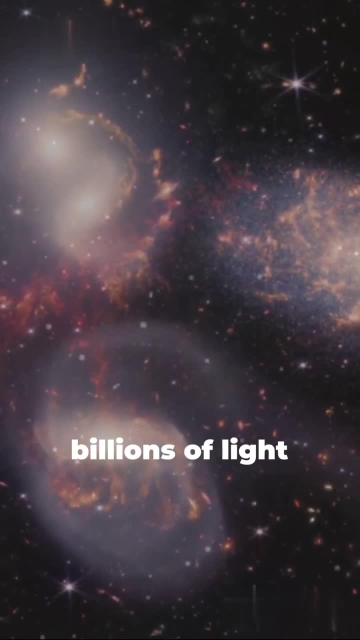 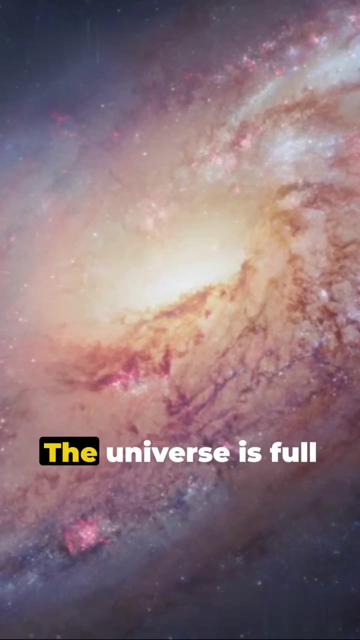 our window to the high-energy universe, revealing secrets that lie billions of light-years away. Every second, every minute, it's there tirelessly mapping the gamma ray sky. The universe is full of mysteries and the Fermi Gamma Ray Space Telescope is helping us solve them. one gamma ray.